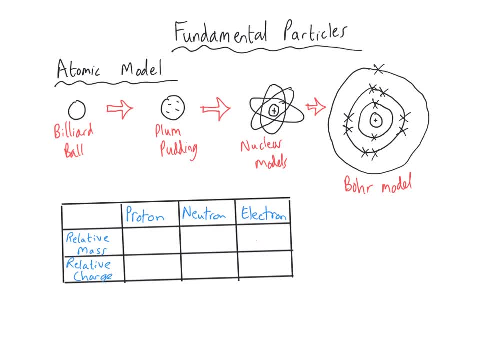 Ball model of the atom and that consisted of the electrons arranged in energy levels. So the nucleus of the atom contains the protons And neutrons, and these are held together by what's called the strong nuclear force, which is a, as the name suggests, the strong nuclear force is a very, very strong force. 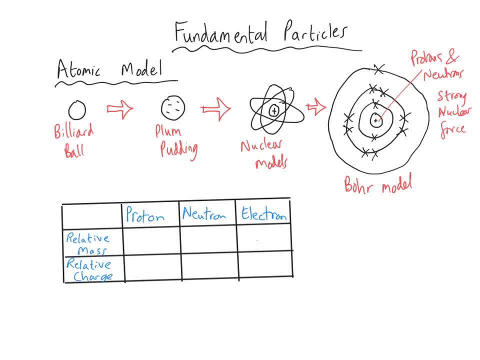 So the nuclear force is a very, very strong force, Far stronger than the electrostatic attraction, which is what we get- that holds these electrons in place around the atom. This is the electrostatics, and the nuclear force is much stronger than the electrostatic force that holds these electrons into place around the atom. 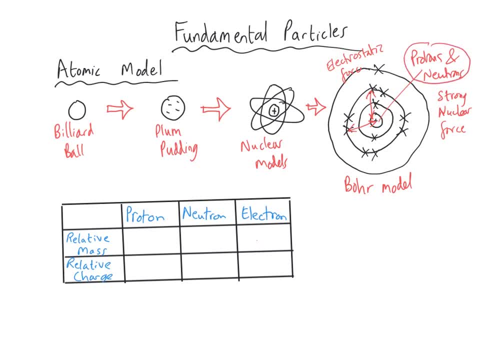 And so these protons and neutrons are held together by the nuclear force and they are referred to as nucleons. So the things in the nucleus Are referred to as nucleons. When we look at protons and neutrons and electrons, they are absolutely tiny. 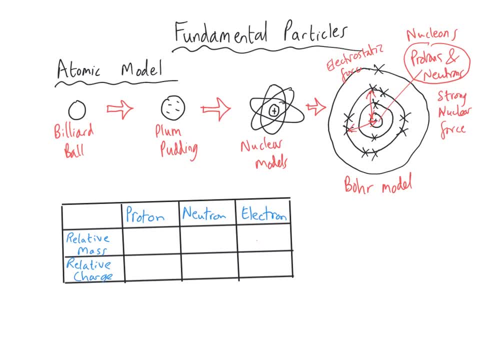 And so when we're thinking about how big they are, we don't look at their actual mass, because the actual mass of a proton is something like one point six, seven times ten to the minus twenty seven kilograms, And their charge is even smaller in terms of the coulombs of charge. 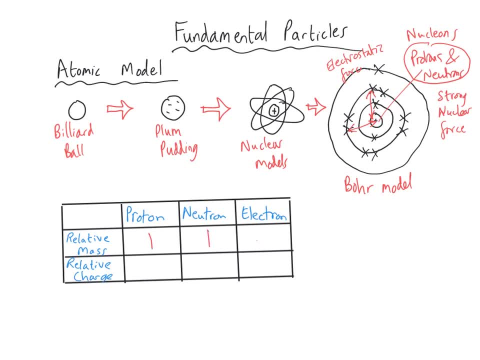 So we compare them and we say a proton and neutron, They've got the same relative mass and we give that a mass of one. And when we compare it to electrons, electrons are almost zero, but not quite. It is one over one thousand eight hundred and forty. 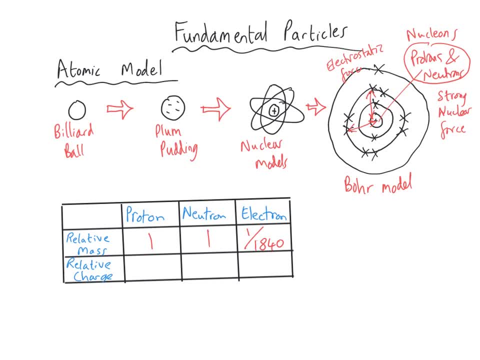 So we need one thousand eight hundred and forty electrons to equal the mass of one proton. That's what that means in terms of charge. Protons have got a massive charge of plus one and electrons have got a charge of minus one, which is why in an atom, the number of protons 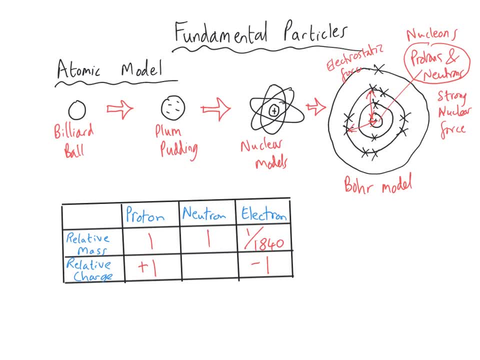 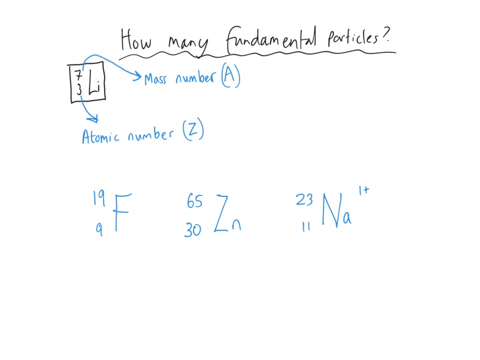 And the number of electrons are the same, because we end up with no charge overall, because the protons and electrons are equal in an atom And, last of all, neutrons are neutral. Neutrons have zero charge. If we move on now to have a look at how many fundamental particles there are in atoms- or ions, depending on what we're looking at- 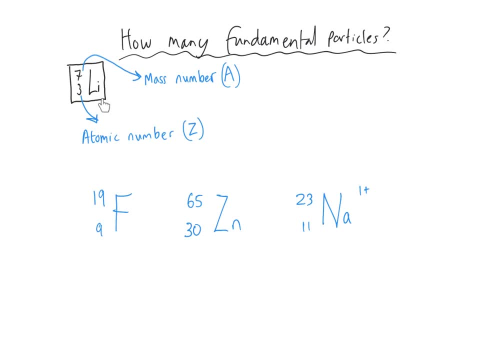 We need to have a recap of how We can use the periodic table to help us do this. So remember, all elements have got their own symbol and then they've got some numbers. everywhere Elements got two different numbers. The numbers are called the atomic number, and that is given the symbol Zed. and we've got the mass number, which is given the symbol A. 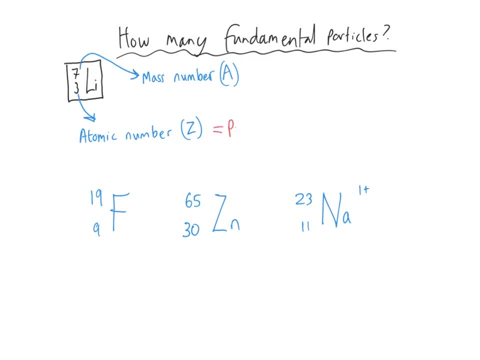 Now, the atomic number is the number of protons in an atom, and the mass number is the number of nucleons. That means the number of things in the nucleus, And so it is a number of protons plus the number of neutrons. 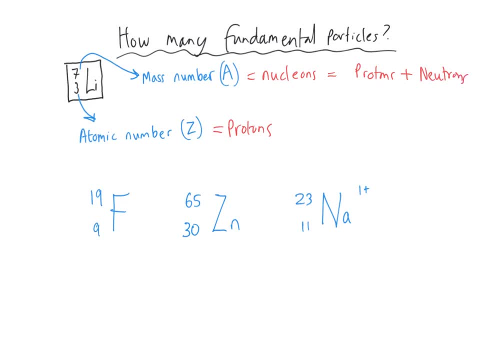 So it's the sum of those two values. So if we have a look at fluorine down here, in terms of protons, fluorine will have nine. Now we said on the previous page that for atoms the number of protons and the number of electrons is the same. 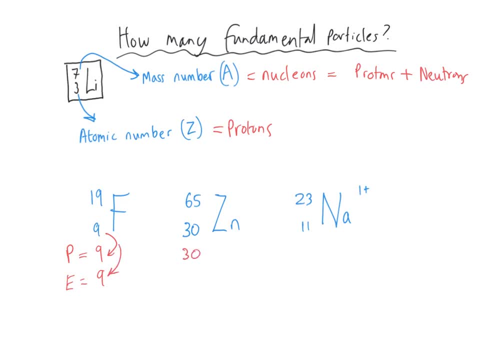 So that nine will be for both of these. Zinc will be exactly the same, Nine protons for fluorine, Thirty protons for zinc, 30 electrons as well, Where we'll get some differences over here for sodium, because that 1 plus tells us that sodium is an ion And more specifically, it is an ion because it has lost. 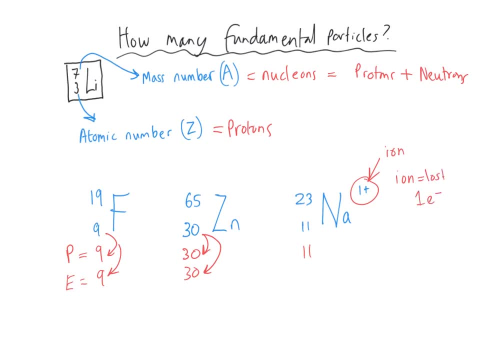 one electron, And so what that means is it's got 11 protons, because that's its atomic number, but it will only have 10 electrons this time because it has lost one. Now, if we have a look at neutrons, the neutrons is the total number of protons plus the number. 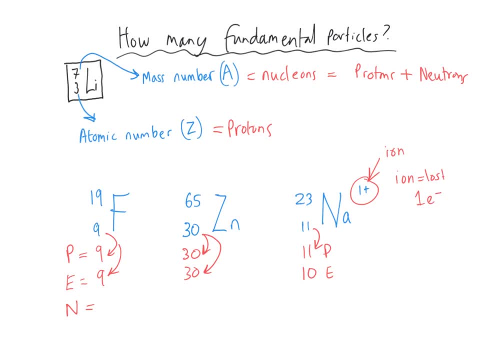 of neutrons. So if we've got nine protons in fluorine here and we've got an atomic mass of 19, a mass number of 19,- then the number of neutrons can be found by doing 19 take away 9,. 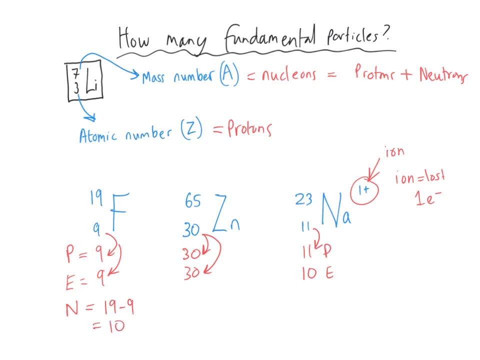 which is 10.. And we can do 65, take away 30,, which is 35 neutrons. And here the number of neutrons is 19.. And we can do 65, take away 30,, which is 35 neutrons. 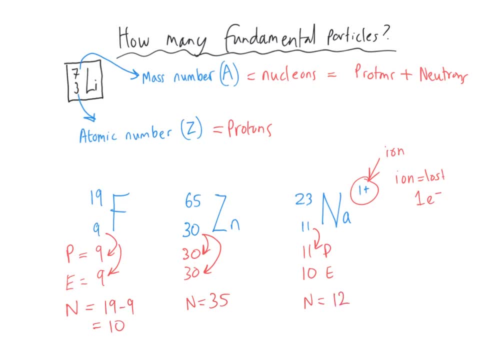 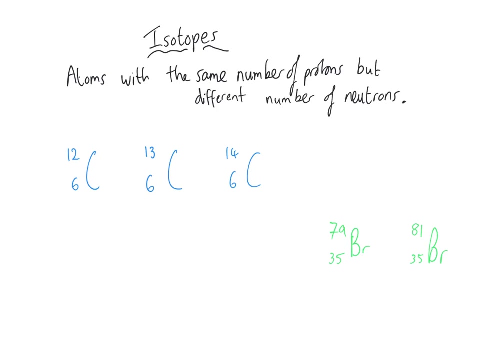 It's 23, take away 11, which is 12 on there. So the neutrons is the atomic mass number. take away the atomic number over there, the big number, take away the small number on there. We're going to have a look now at some more complicated particles called isotopes. 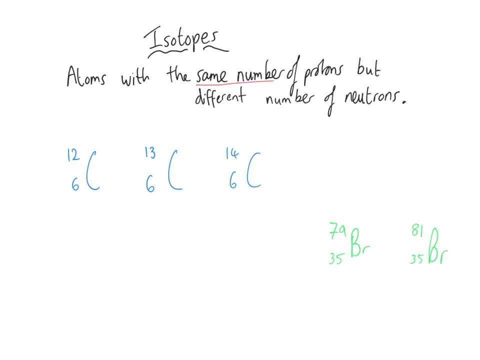 Now isotopes are particles that have got the same number of protons but different numbers of protons. So we're going to have a look now at some more complicated particles called isotopes, And so I've got some examples here for us to work out. So the protons in these substances 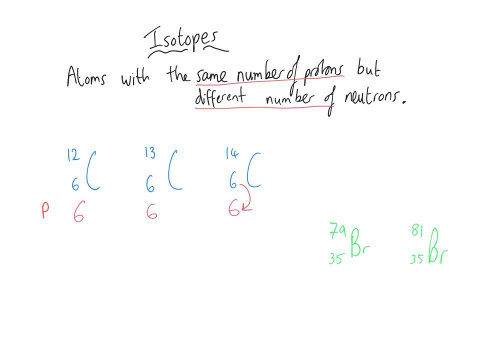 nice and easy: six for all of them, because the atomic number is six every single time. The electrons is also six for every single one of these, And the neutrons this time is going to be different: 12 take away six is going to give us six neutrons for this one. 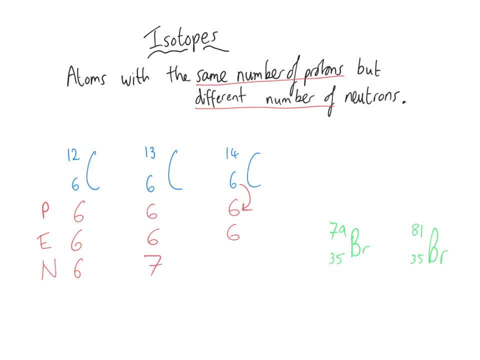 13- take away six is going to give us seven neutrons on here, And 14- take away six is going to give us seven neutrons on here, to give us eight. If we have a look at bromine down here, bromine has got 35 protons in both. 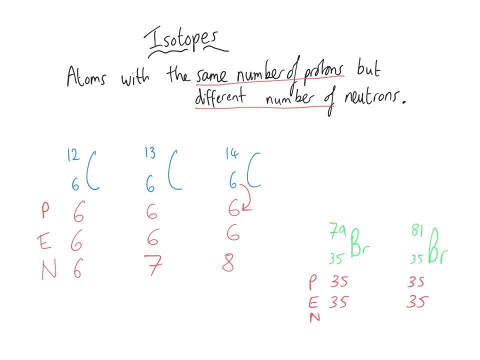 cases. it's got 35 electrons in both cases and this one is going to have 44 neutrons and this one is going to have 46 neutrons. on here Now, a really important thing about isotopes is their reactivity, and actually reactivity is governed by the one particle which isn't mentioned in the 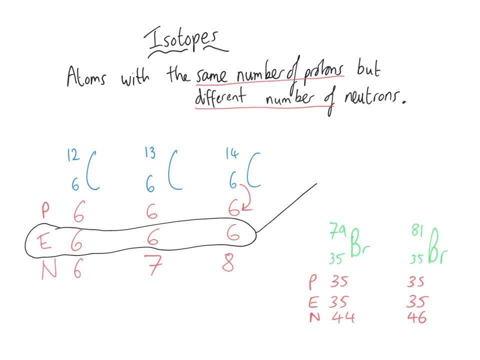 definition of what isotopes are, which is electrons, And the fact that these three isotopes of carbon have all got the same number of electrons, they will react in the same way chemically, irrespective of the fact that they're slightly different masses on there, And the same would be. 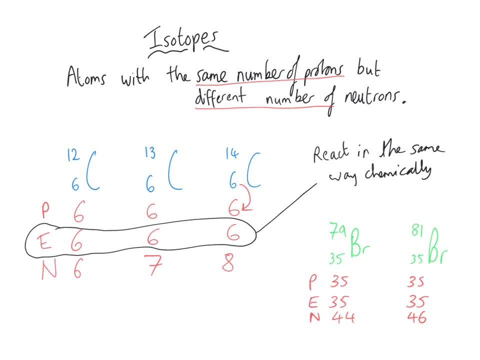 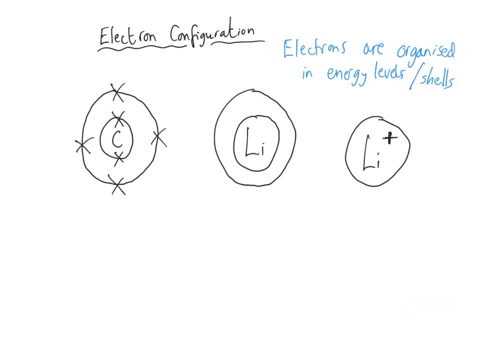 true for the bromine. those two bromine atoms would react in the same way because they have both got 35 electrons. We're going to move on now to have a look at electron configuration, which is a fancy way of saying: how are the electrons organised around the nucleus of an atom? Now we know at GCSE that these 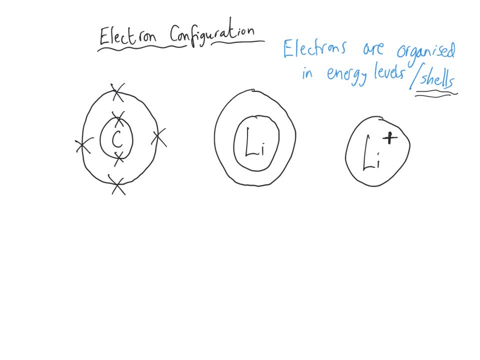 are organised in shells, and you might have also called them energy levels too, and we'll find out later why we bother calling them energy levels instead of shells. Now for carbon. carbon has got two electrons in the first shell and it's got four in the second shell, So simple electron. 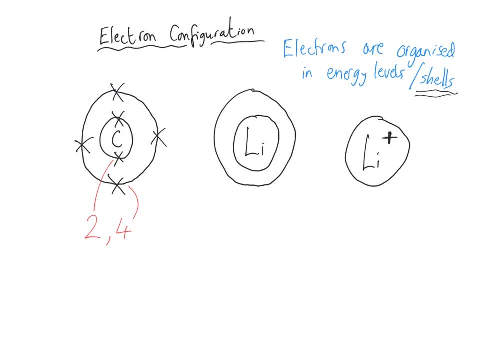 configuration sort of GCSE level would have had, was listing them as 2, 4.. Now lithium, which has got three electrons, would put two electrons in the first energy level, or shell, and one in the second one, and the electron configuration would be this Lithium plus, which once again is an ion. 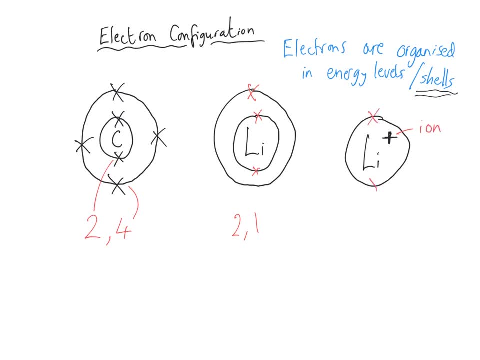 it's positive still, so that means it's lost an electron. it would have only two electrons, and so its electron configuration would be two, with a plus like that. Now this idea has evolved into a more sophisticated model, mostly because we discovered that electrons in a particular energy 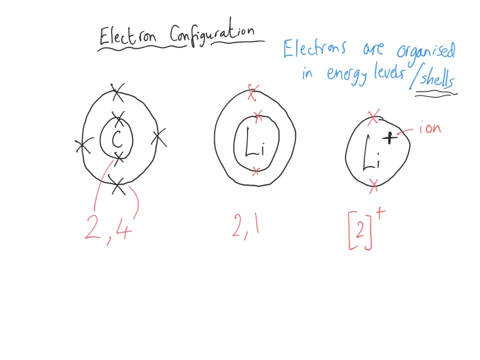 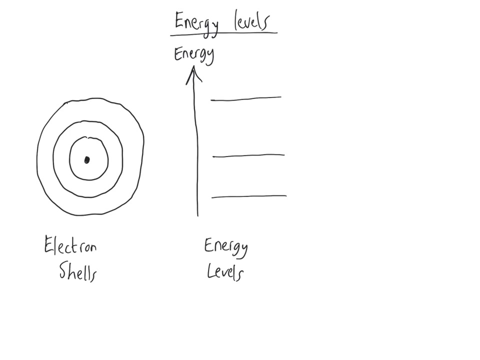 level are actually not all the same. Now, at GCSE level, you're keeping the model simple. so this is what we've considered so far, but what we're going to move on to now is looking at the slightly more complicated model. So, first up, if we consider the electron shell model, again, we know that the 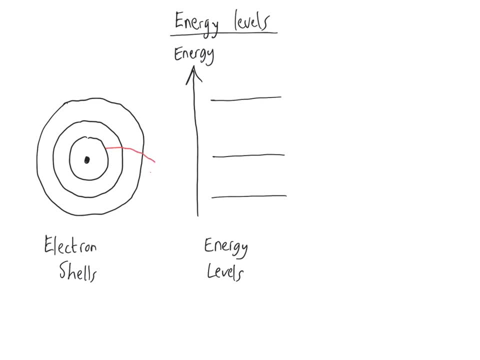 second shell can hold two electrons and the second shell can hold eight electrons. Now, what you were not taught at GCSE level is actually: the third shell can hold 18 electrons and not actually eight, which is what you were taught. But what we were careful to do is only consider. 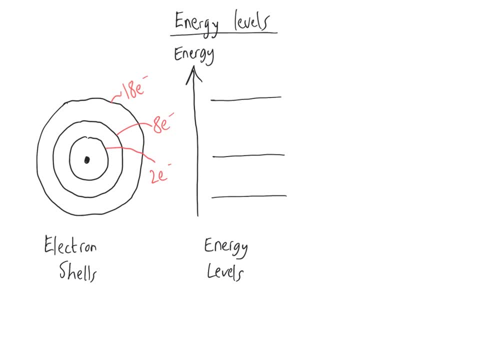 the atoms up to number 20, and so this rule, this extra complication, didn't actually come up. it wasn't an issue on there. Now, the electron shells that we've just been looking at, the first, the second and the third- 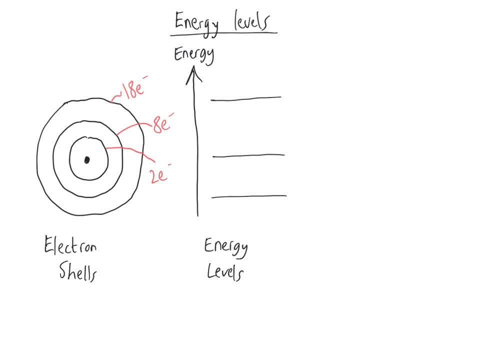 they will all have different amounts of energy because of how far they are away from the nucleus. The first electron shell has got less energy than the second, and that has got less energy than the third, and that is why we can call them energy levels instead of shells, because the first shell 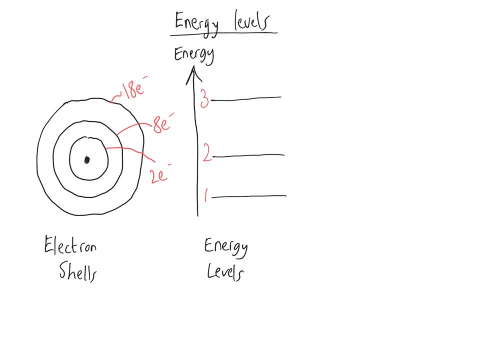 has got less energy and the second has got a higher energy level and the third is a higher energy level. Still, this gets even more complicated because electrons in different shells have got different amounts of energy, and so we can take our energy level diagram and actually add an extra level of. 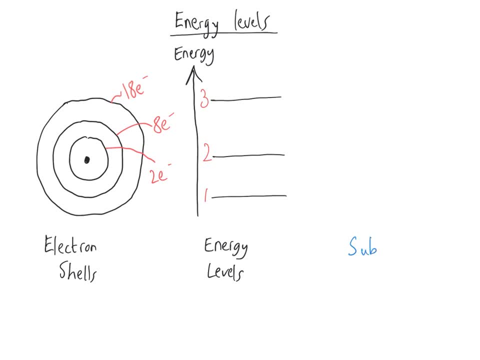 detail to it. Instead of just looking at energy levels, we can look at sub-levels, sometimes also called sub-shells. Now, the first one is nice and easy. The first sub-level is the same as the first energy level. but it immediately gets complicated after that first level because 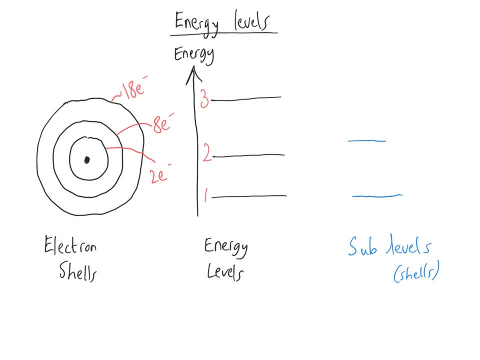 these levels are divided into the sub-levels, which have got different names, and their names are S, P, D and F. They don't all have all four of those different names, but they do, starting from the second energy level, start to have some variety. So in the second energy level, 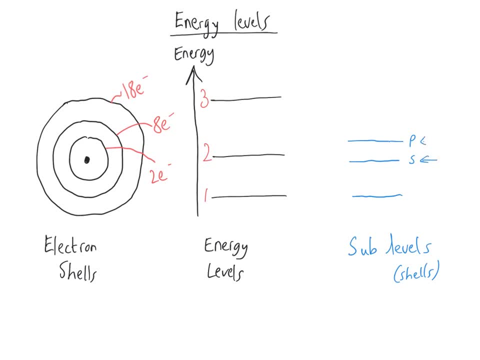 we've got the S sub-level and the P sub-level, and they've got different amounts of energy, and so the electrons in the second energy level aren't all the same. The electrons in the third energy level aren't all the same either. We've actually got three sub-levels on here. We've got 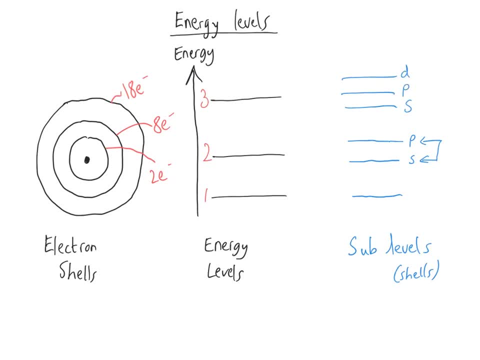 the S, we've got the P and we've got the D sub-levels on there. And just to go back to the number of electrons that an energy level can hold, there's actually a rule that you can remember: where the number of electrons is equal to 2n squared, where n is the number for, 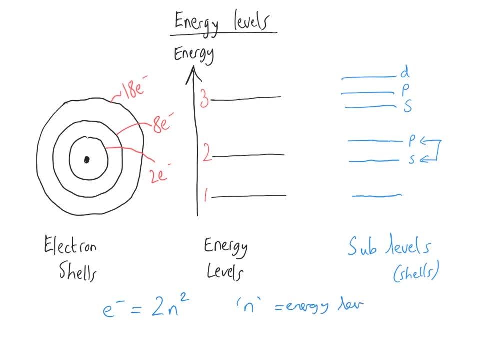 the energy level, And so what that means is that if we are in the second energy level, we've got two lots of n squared. So 2 times 2 is 4, then times by 2 again gives us our 8 that we have in the second energy level, And for the third energy level we've got 3 squared. 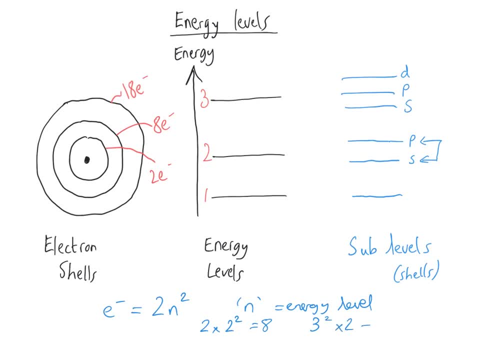 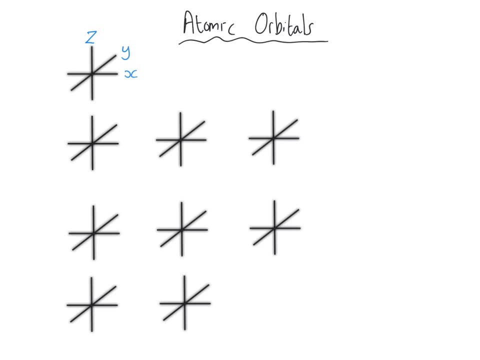 because it's n squared, which makes 9.. We're then doubling it, which makes us our 18 electrons that we can have in each energy level. We're going to look in a bit more detail now at what sub-levels are actually like, And before we can do that, we need to recognise, in fact, that 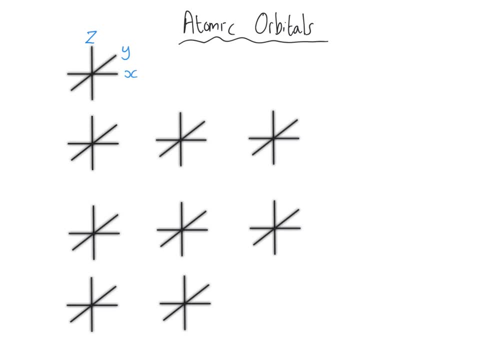 electrons as we know it at GCSE, we don't quite consider them in the same way. We don't consider them to be a particle anymore, but a cloud of negative charge, And an electron fills a particular volume of space called an atomic orbital, And different atomic orbitals have got different. 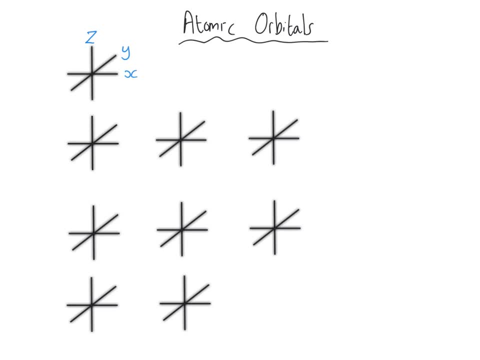 energy levels, And each atomic orbital has got a number that tells us what energy level it corresponds to, So that might be a 1 or a 2 or a 3.. But the atomic orbitals have all got different shapes as well, which in turn have got slightly different energy levels And 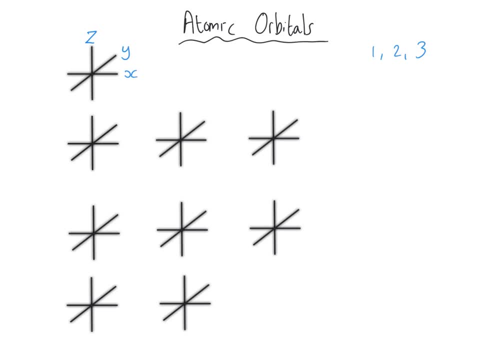 these are called sub-levels that I've mentioned before, And we refer to these as S or P or D or F, And these orbitals have all got different shapes, which I'm going to have a go at drawing now. S orbital is actually just a spherical shape, So that's nice and easy to remember: S for spherical. 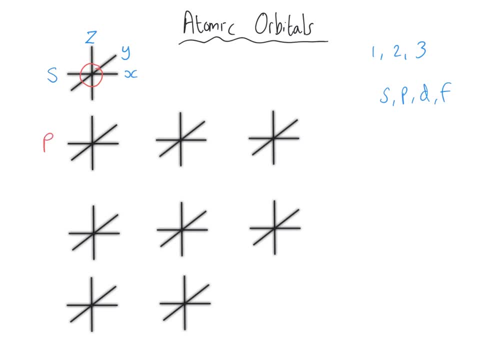 The next ones are P orbitals. Now, P orbitals, there's actually three different types of P orbital, And they each follow one of the X, Y and Z planes on here. So that's a PX orbital, And then we've got a PZ orbital that goes on the Z axis up there, And then, last of all, 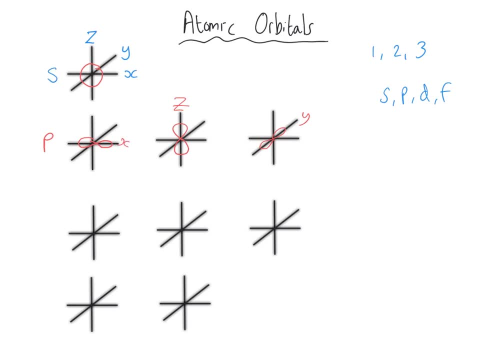 we've got a PY orbital on there. So those are three different P orbitals that we've got, And then the last type of orbital that you need to be aware of is the D orbital. Now, they're really complicated to draw, So I'm not going to draw them whilst doing this. 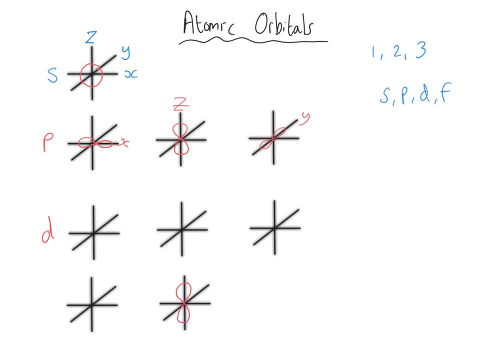 video, but except to do one which is my favourite, one, which is where we've got one part of the orbital goes up the Z axis and then another part sort of circles around like a hula hoop over there. But just we need to know that there are five different D orbitals on there. 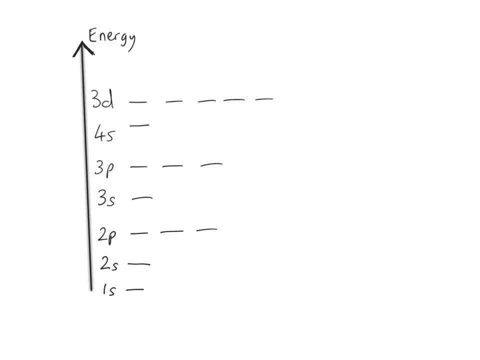 Now let's take a look at these. So we've got three different types of orbitals represented in our energy level diagrams. As I said before, the first energy level consists of a single S orbital, And that's what we're showing on here, And the second one is split into 2S and 2P. 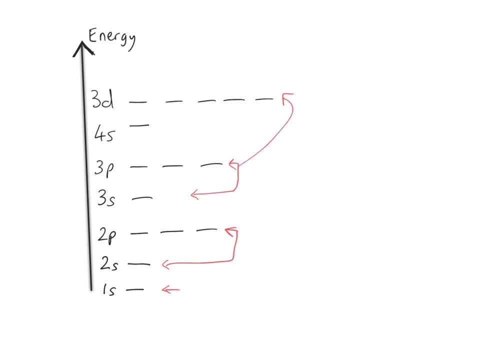 And then the third one is split into 3S, 3P and up here, 3D. on here, Now we've got some rules that we need to recognise. So first up, each atomic orbital can only hold a maximum of two electrons. 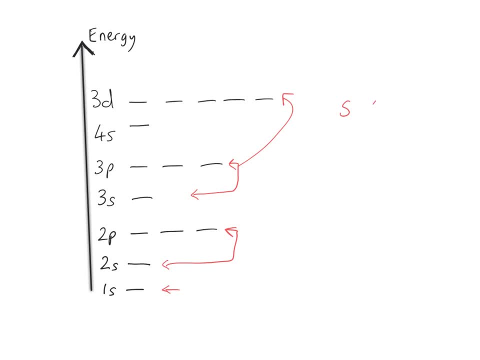 And the S orbital. since there is only one orbital in the S sub-level and each one can only hold two electrons, then the number of electrons in total in an S orbital in the S sub-level is two In the P sub-level, because there are three different orbitals in the P sub-level, as we can see down here. 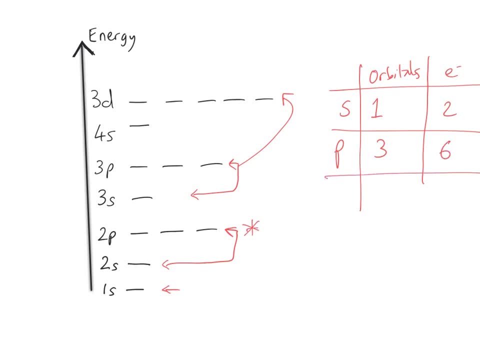 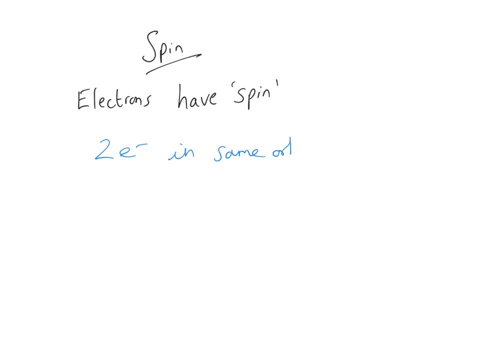 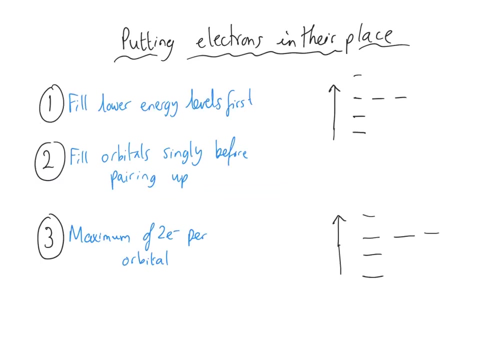 in the same orbital and they have got opposite spins, and what we do to represent that is we use arrows and we use one arrow up, we call that spin up, and we have another arrow pointing down and we call that spin down. now let's have a look at how we put electrons into their places. 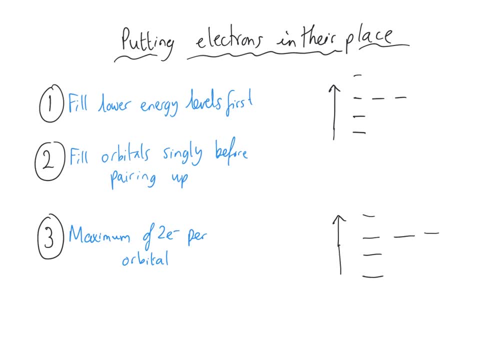 around the nucleus of an atom. so there's three rules here. mostly there's two rules, but i've called it three. so the first rule is that you must always fill the lower energy levels first, and that's because the lower energy levels are more stable and that's where they will go the 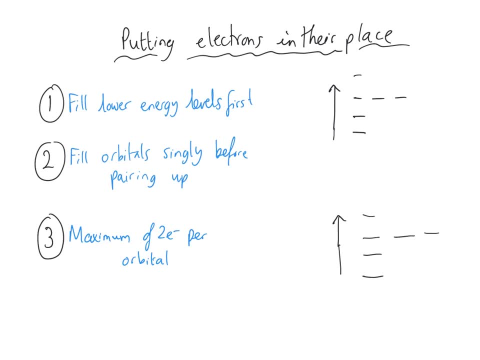 electrons. the second rule is that when you're putting electrons into orbitals, you fill them singly before you pair them up. so that means you put them in one at a time, and then there's rule three: you fill them in one at a time, and then there's rule three, you fill them in one at a time. 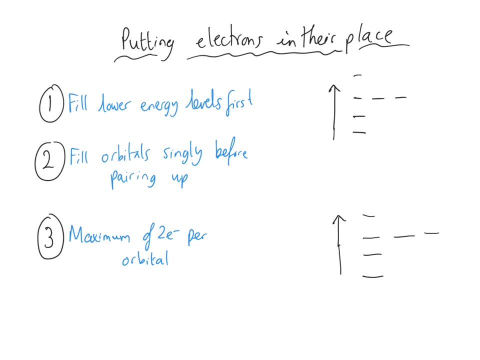 which is just a reminder rule, really, which is that you put two electrons into an orbital and then it is full. now let's have a look at an example on here. if we consider first of all carbon, which has got six electrons to put in, we've got the one s sub shell. we put two electrons into there. 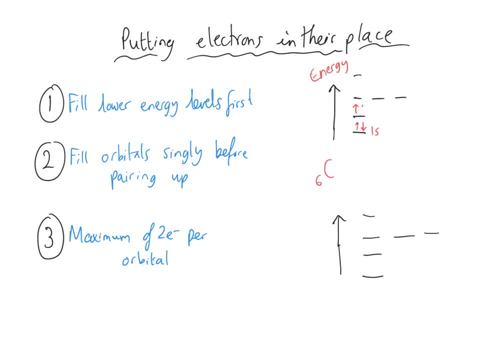 and then it is full. we've got four more to put in, so we put two into the two s sub level and then that is full. and then, last of all, we've got two more electrons and we put them into our two p sub shell. on there we don't need to fill that up, and if we have a look at, 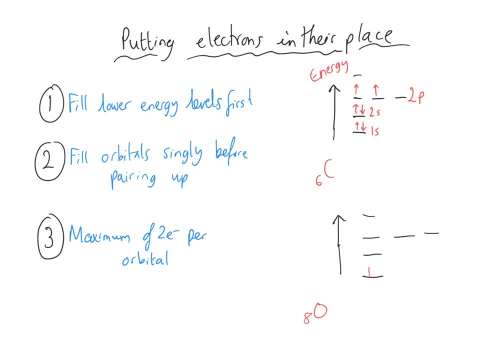 oxygen, which has got eight electrons. it's the same thing here with the one s, the same thing here with the two s, and then when we get to the two p, because because we've only used four electrons down here, we need to put another four into the two s sub level on here, and so we've put three in. 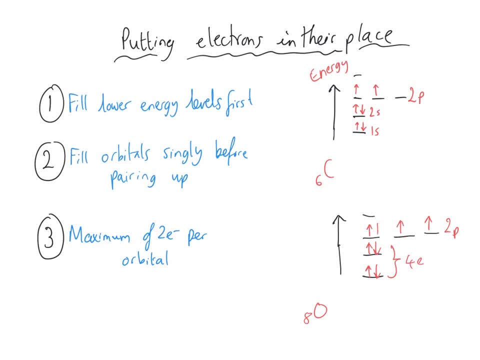 and that's our single occupancy, and so we don't have a choice. now we're going to put the two s into there and we get this double occupancy, which does affect the quality of oxygen. that we'll come to later. we can write the electron structure or configuration in a similar way, but more complicated. 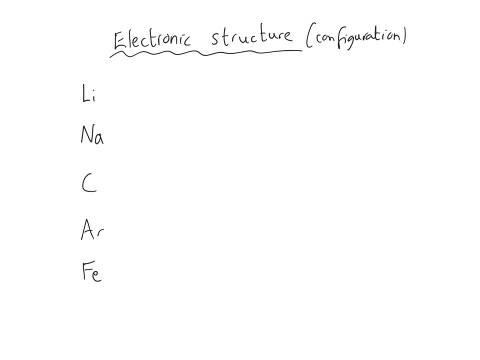 so we were doing a gcse level. so lithium has got three electrons and so we need to put those into their sub levels. so the first two electrons will go into the 1s sub level and the second one will go into the two s sub level and the third one will go into the two s sub level. 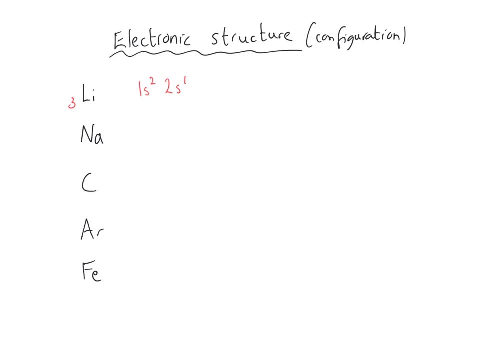 and the second sub level is now needed to have one electron in it and that is now full. what you've got is you've got the powers in a way, because they're always up in the air numbers, they're not down on the line that is equal to the total number of electrons that we've got in our 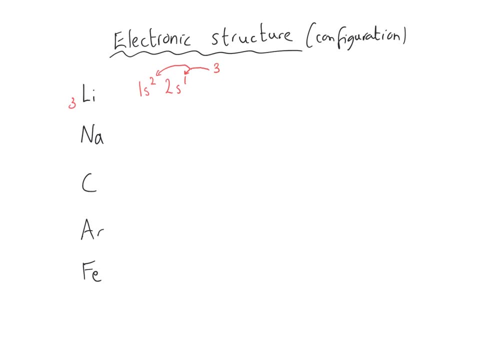 particular atom. so three for lithium on here, and if we have a look at sodium, which has got 11 electrons in total, that will be 1s2, then that's full 2s2, then that's full 2p6 and that's so far. if 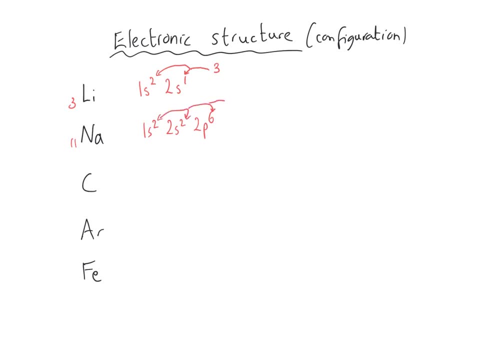 we're keeping track is two and two and six, which makes ten, which means we need one more electron, and 3s1 gives us our 11 electrons in total. for carbon, we have got six electrons. so we write 1s2, 2s2, 2p4 and that's then done. we don't need to do all this up here. this was just me keeping. 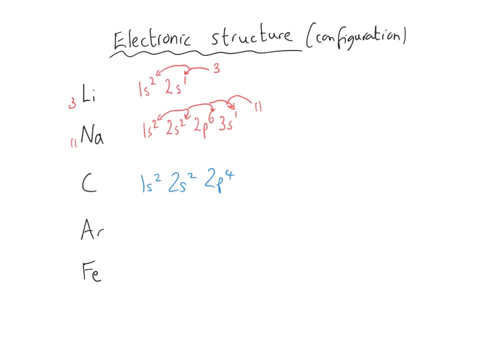 track of the total number of electrons for you. you don't write that in the electron configuration argon argon's actually got 18 electrons, so that's a little bit lengthier. and that's the first 10 electrons done on there, and then the next two, and then the next. 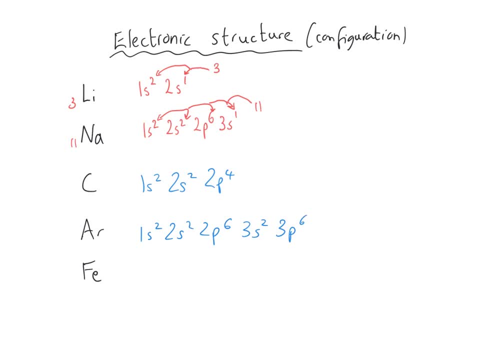 six and that's done on there. that's a total of 18 electrons on here. iron has got even more electrons- it's got 26, and so the first 18 will be exactly the same as argon, so no extra thought needed on there. and then we've got another eight electrons to put in. 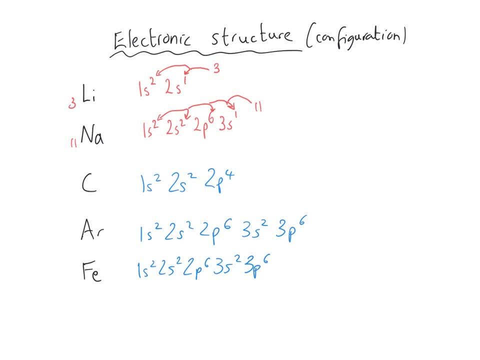 and so we need to get to that rule where you fill the 4s electrons before you fill the 3d. so we've got 4s2, 3d6 on there, and that's our total number of electrons now, even though we fill the 4s before the 3d. what we should really do, though, is we should not have 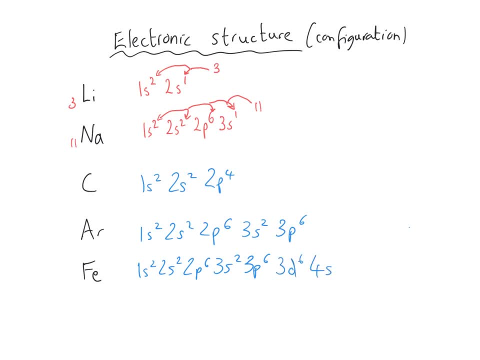 the 4s first. we should have the 3d6 first and the 4s too, because a as soon as they become occupied, the 4s actually gains a little bit of energy, which causes an issue that we're going to come across in just a moment. Last of all, to do with these electron. 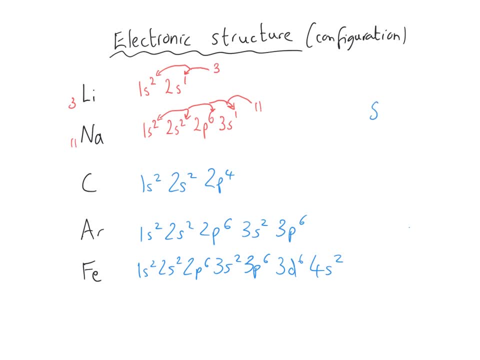 structures, electronic structures. we can indicate something about our elements that we have been looking at and we can refer to them by the identity of their outer electrons. So lithium and sodium are referred to as S-block elements because their outer electron is in an S-level. 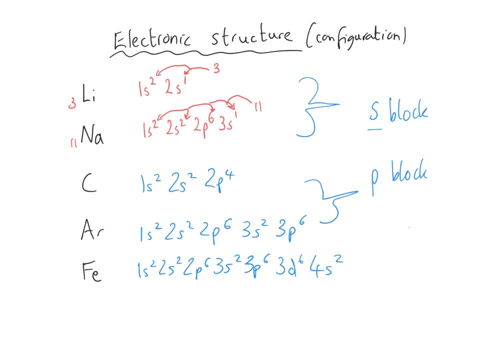 and carbon and argon are referred to as P-block elements for the same reason Their outer electrons are in a P-level. Iron is referred to as a D-block element because its outer electrons are in a D-level. It's got an intensity of an electron, So it's got an intensity of an electron, So it's got an intensity of an. 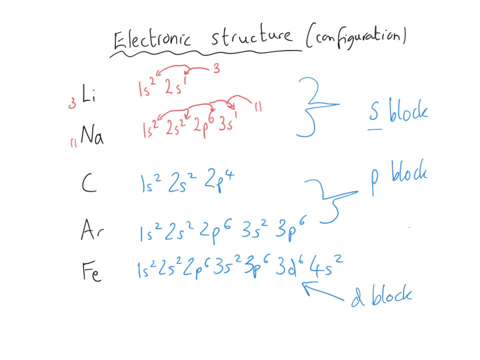 incomplete D sub-level, which is one of the characteristics of the transition elements, And you can navigate your way around that by looking at the periodic table, because the S block is everything in group 1 and group 2, the P block is group 3 to group 8, and then the D block. 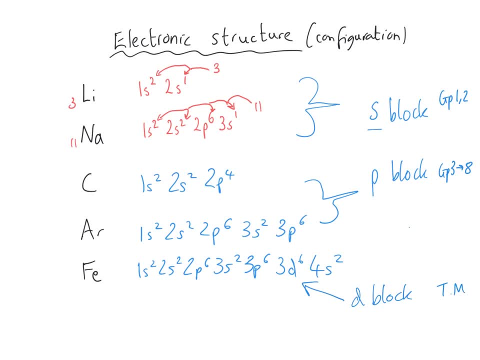 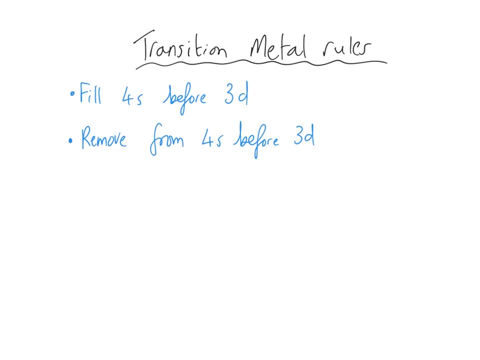 is the transition elements on there or the transition metals they're sometimes referred to. Now, as I've already said about transition metals, there are two rules about the transition metals. You always put the 4S electrons in before you put the 3D in, although you do usually write. 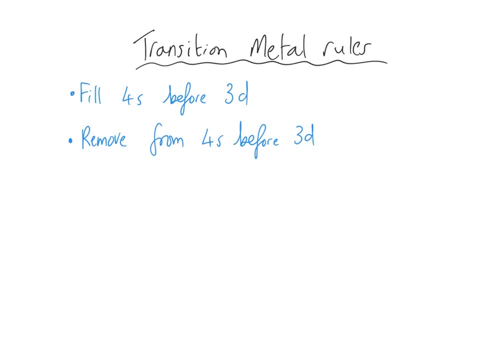 the 3D first, as you're listing them, and then you remove the electrons from the 4S before the 3D. so that's relevant if you're working out the electronic structure of some particular transition metal ions. There are two exceptions to the. 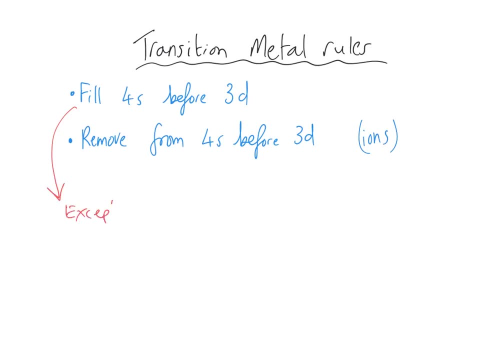 fillings of the transition metals, and one of them is the transition metal ions. There are two filling rules that you need to be aware of, and those exceptions are for chromium and for copper. So you would expect chromium to have the electron structure 3D4, 4S2,. 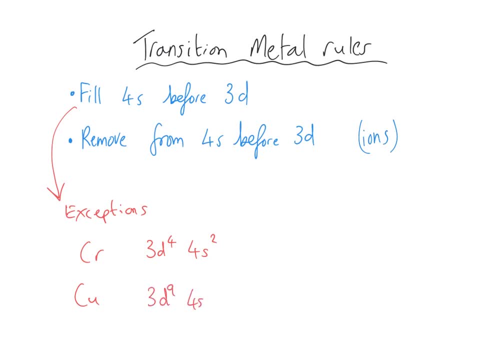 and you'd expect copper to be 3D9, 4S2.. But actually that's not right, because chromium and copper would get more stability if they do something slightly different. And what they have is they have 3D5, 4S1 for chromium and 3D10, 4S1 for copper, And that precisely full. 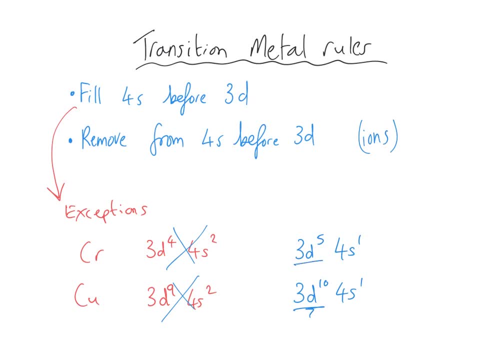 D energy sublevel, and that half full D sublevel gives the elements extra stability that they wouldn't have if it was almost full or almost half full. So these are actually more stable, and so this is the organisation that we get. So we have a lot of different fillings that we can use for chromium and for copper in terms of 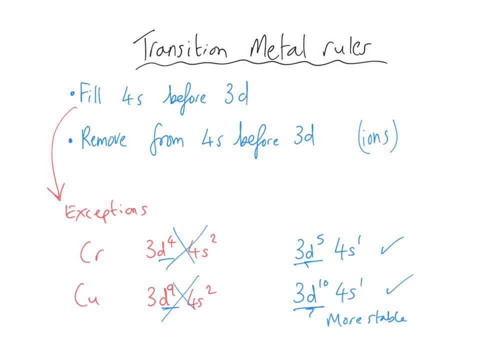 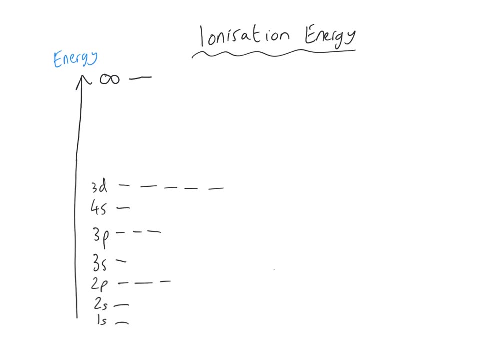 their electrons. and those are two exceptions that you need to know of. Now let's have a look at ionisation energy. The ionisation energy: obviously it's the amount of energy, because that's in its name, but it's the energy required to remove one mole of electrons. 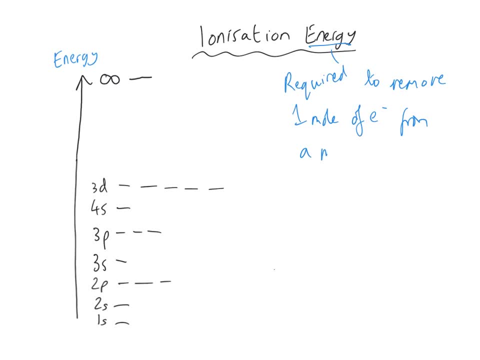 from a mole, There are lots of elektron. so at this, what does that actually mean? Well, what that means is the electron that gets removed is no longer a part of that atom anymore. So if we just consider something simple and small, let's do lithium- There it's got three electrons. 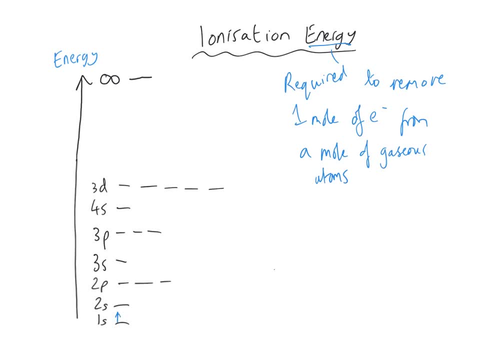 if we're going to ionise lithium, we have to give lithium more energy to get this electron, to nämlich get the electron small enough in this personaje space to make it smaller. Come on, the liquid can't get smaller. we can't get it bigger than a mole, so in this case it's bone and just turn everything green. you can't get 복istein in lithium, so what we're just going to. 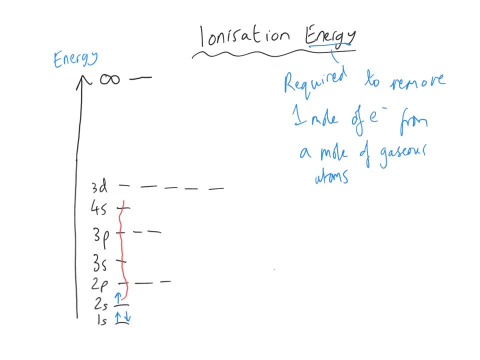 to jump, not just up a few sublevels or a few energy levels, but we actually have to get it to jump so far that it has left all the energy levels behind. So we've given it enough energy to make that leap from what's called the ground state, where the element has its electrons. 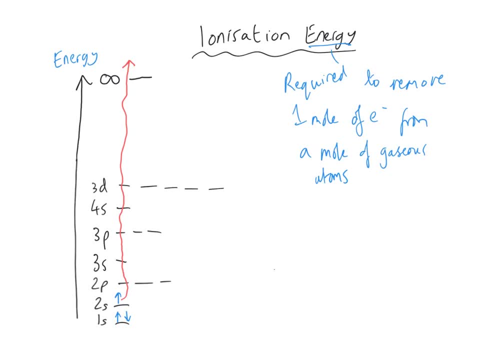 normally to those electrons aren't part of that atom anymore And this energy level- infinity- that's kind of considered to be the outside of the atom. So when you're ionising something, you're giving the electron enough energy to leap from where it normally is in the ground state. 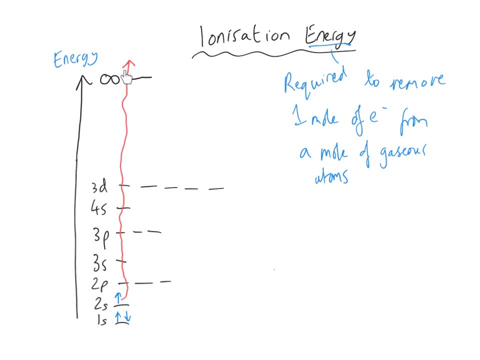 past all the other energy levels, past the outer energy level, and it's gone. And so that's the ionisation energy of a particular substance, And what you can see from this diagram is if something's outer electrons was in a D sublevel. 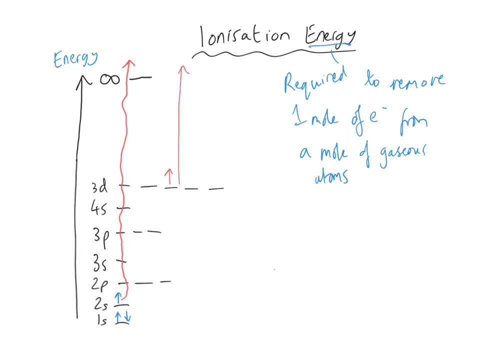 the amount of energy needed to make that electron leave the atom actually wouldn't be as much energy as if it was down here in the 2s, because that amount of energy, that energy change, given the symbol delta E, is obviously different depending on if you're in a higher energy like 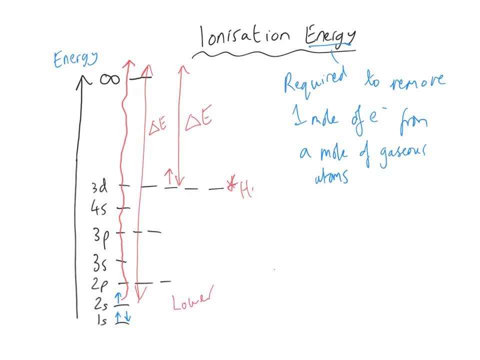 this one, or a lower energy like that one, And so ionisation energy varies from atom to atom. And these numbers that we have, they're all measured with the units in kilojoules per mole of that substance. Kilojoules per mole. 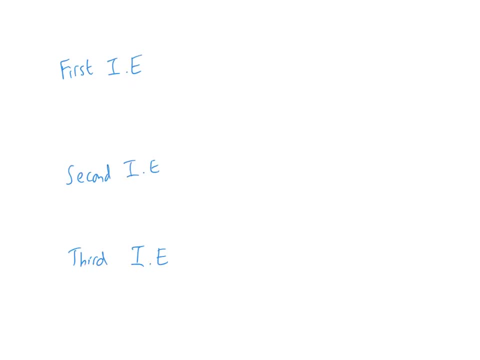 In terms of ionisation energy. I was just looking at taking one electron away from a particular element, but you don't always have to limit it to one electron. You might take away more than one electron. Now, the first electron you take away is called the first ionisation energy. 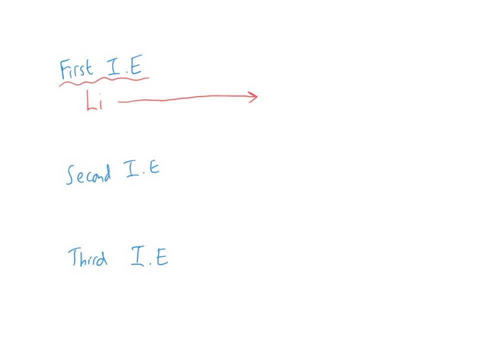 And the equation that you have to write to represent the first ionisation. energy always has the element on the left-hand side. The element has to be in the gaseous state and then it turns into an ion which is also in the gaseous state, and we lose. 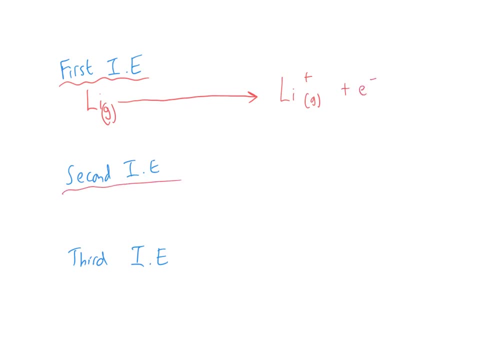 an electron. So that's the first ionisation. The second ionisation, energy, is. very logically, you've taken one electron away, and so you've got your gaseous ion. We're going to take another electron away from it as well, to leave us with a gaseous ion that has lost two electrons, and so 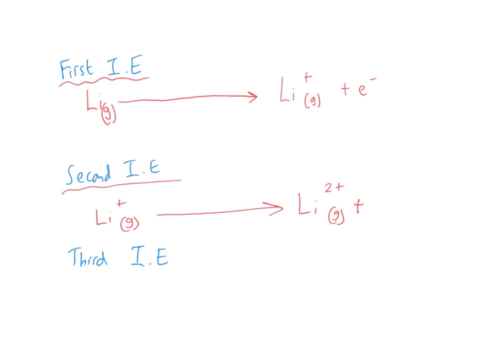 is therefore a two-plus ion and we get our final electron on there, just the one electron on here. And last of all, for my examples, the third ionisation energy. we take an ion that's already lost two electrons, so it's a two-plus ion. it loses another electron and so it becomes a three-plus. 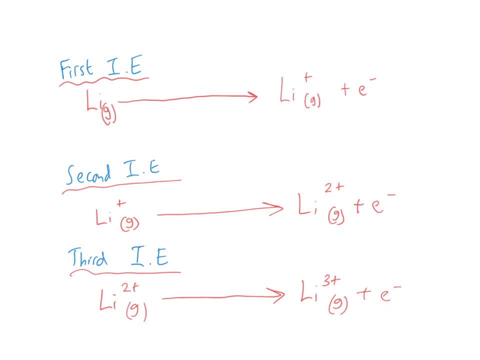 ion, this time losing another electron. In terms of comparing these ionisation energies to each other, the first ionisation energy is always the smallest number, and that's because we're taking an electron away from a neutral atom. Then the second ionisation energy is larger than the first, and that's because the electron 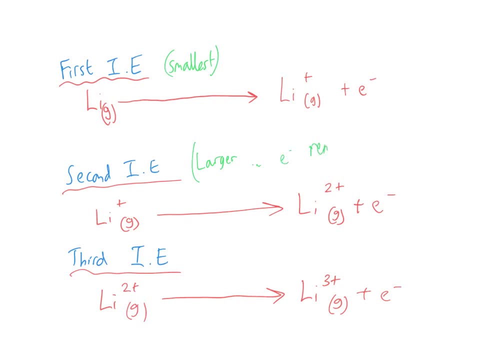 is being taken away from some of the other electrons, So we've got a two-plus ion, and so we've got something that is a positive ion. and so what that means is, because it's a positive ion, we've got greater electrostatic forces of attraction. because we've got something that is: 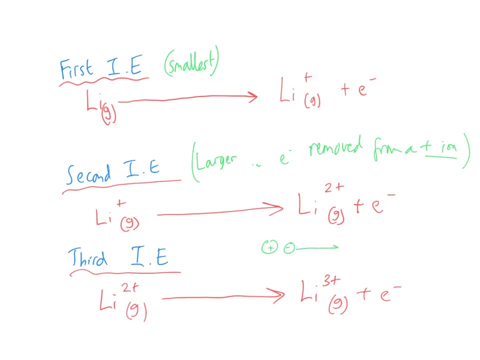 positive and we're trying to take that negative electron away from it and there's really strong electrostatic forces on here And it follows that the third ionisation energy is going to be larger still because we're taking an electron away from something that is two-plus, so it's got. 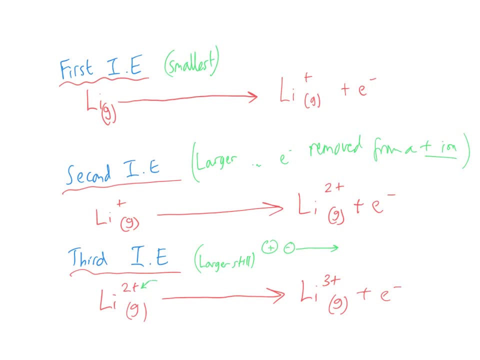 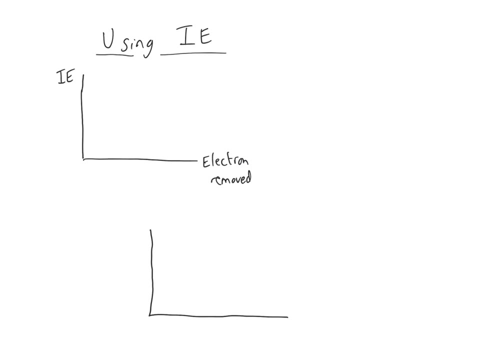 an even stronger positive charge, an even greater attraction for electrons. Now, what can ionisation energy be used for? So the first thing is it provides us with evidence for the electron shell model for atomic theory. And so, if we consider sodium, which has got 11, 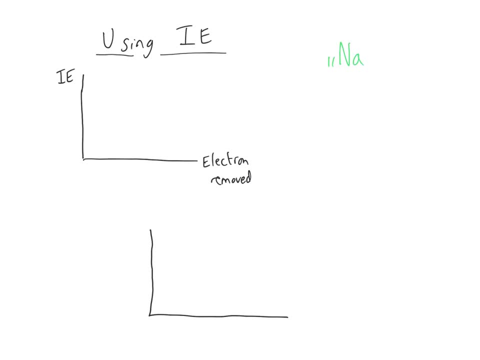 electrons in all of its energy levels. we can investigate what the ionisation energy is for sodium with each successive electron. So the first electron that we remove is really easy to remove. Its ionisation energy is very, very low. The second one is harder. As I've said, you're taking an electron away from something that 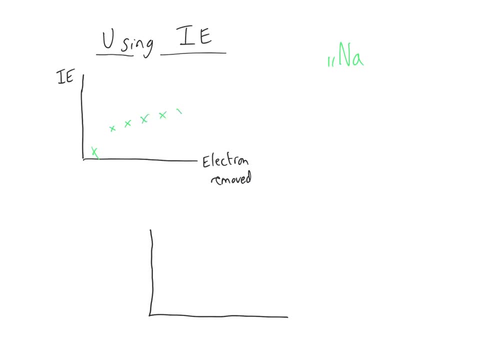 is positively charged. now The successive next eight are all quite similar to remove. It gets a little bit higher, but not massively each time. And now it's easy to see the pattern on here that we've got one electron that's very easy to remove and that's in the third energy level, And then we've got eight. 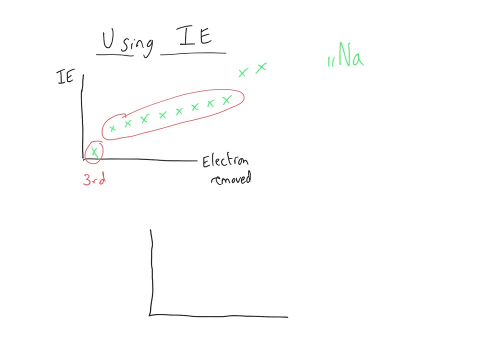 electrons along here, which are reasonably easy to remove, but they get harder as you remove more and more of them, And that's because we're taking electrons from only the second energy level And then the first energy level on here. these are the ones that are hardest to remove. 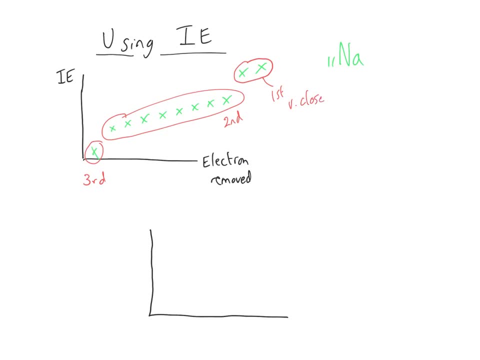 because they are very, very close to the nucleus And so they are experiencing a great deal of energy, And so we can see the attraction from the positive nucleus, whereas as we go down here, this third energy level, these are really, really shielded electrons from the nucleus' pull We've 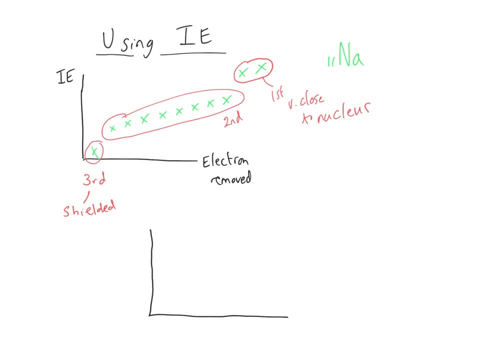 got a lot of different kind of layers in the way, blocking the positive attraction of the nucleus to get to those outer electrons in the third energy level. Now, even cleverer than this is if we consider just the electrons in the second energy level. 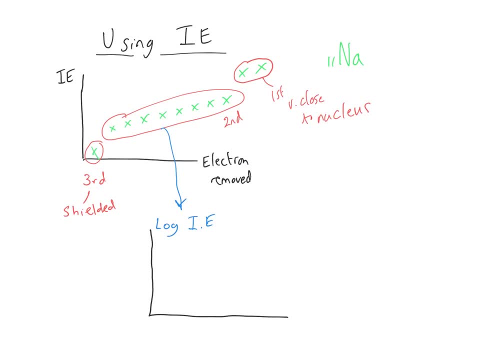 take the log to the base 10 of those ionisation energies and we plot them successively. what we find this time is that we get six electrons which follow a pretty straightforward pattern on their ionisation energy, or log of ionisation energy, increasing as you take one electron, then another. 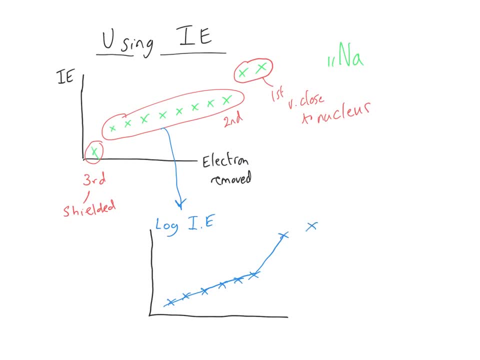 out, But then we get a leap for the final two. So even those eight electrons on here aren't equivalent, and what that gave us our evidence for is that these six electrons that are pretty close together in their pattern they're 2p electrons, whereas these ones on here are 2s. and because the 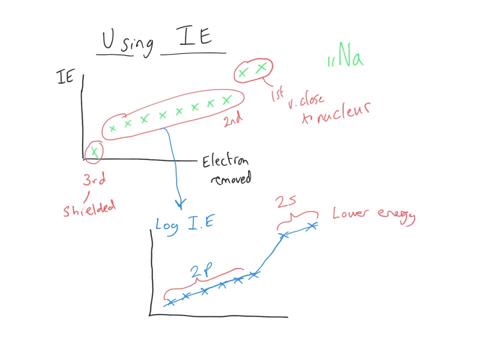 2s are lower energy. what that means is they are therefore harder to remove, because we have to give them more energy to get them to leave the atom. and of course, they're also closer to the nucleus As well, and so that means that they experience a greater electrostatic attraction from the 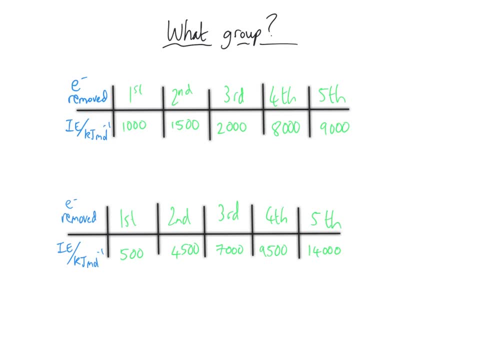 nucleus as well. We can also use ionisation energies to work out what group of the periodic table a particular element might be in. What we have to do to do that is, we have to look at successive ionisation energies, and so if we have a look here, we've got our first element, where the 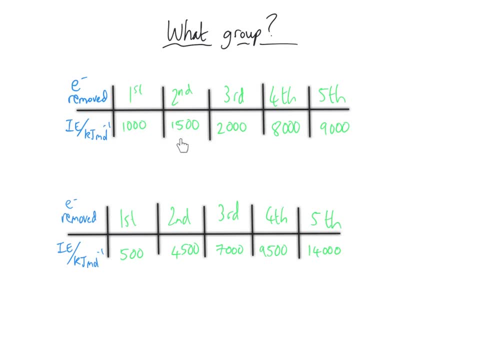 first ionisation energy is the first element of the periodic table. So we've got the first element: ionisation energy is 1000, the second ionisation energy is 1500,, then 2000,, then 8000,, then 9000 and 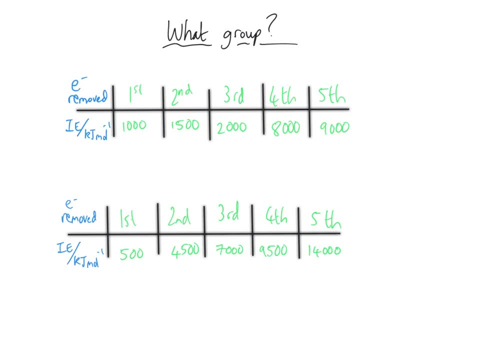 the skill that we have to employ here is: we're looking for a big leap, a big gap, and so for me the big gap here is between the third and the fourth electron removal, and so that means that the first three electrons are pretty similar to remove. as you go along They get a bit harder. but 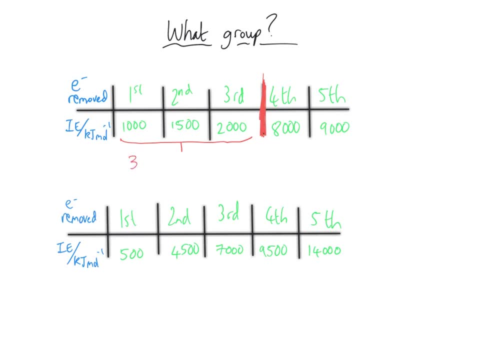 we're expecting them to get more difficult to remove, and so what this tells us is that this has the same amount of energy level- electrons- which therefore means it is in group three of the periodic table, And if we have a look at this next example here for a different element, we can see: 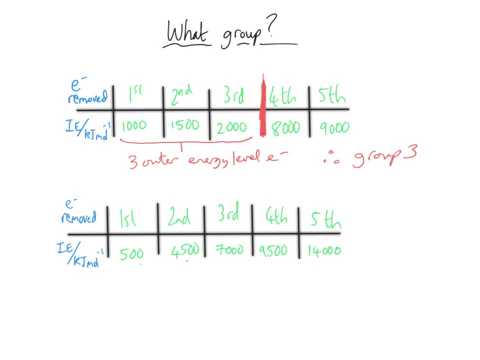 we've got 500, we've got 4500, well, that's a big leap already because that's got nine times bigger. so it's a leap of 4000, it's got nine times bigger If we have a track on here. just looking here, this: 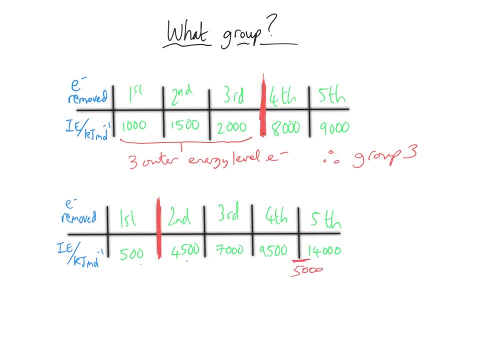 is actually a larger increase of 4500. So we've got a big leap already because that's got nine times bigger. So we've got 5500, but 9500 to 14000 is actually only increase of about 50%, whereas this it got nine times bigger, so that was a much bigger. 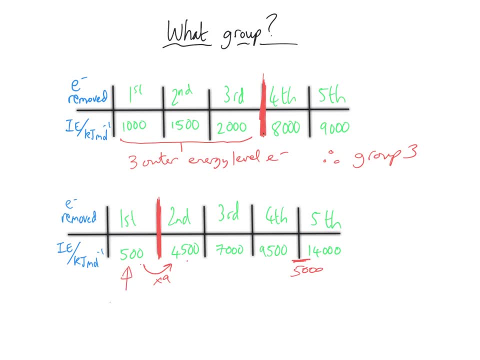 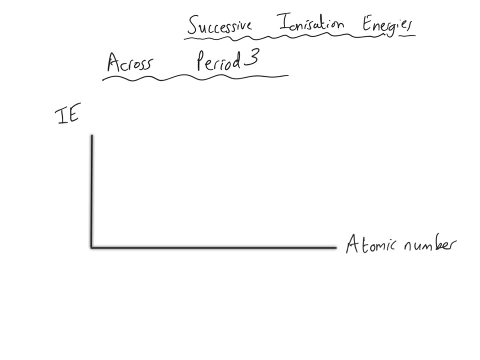 increase on here. So that means that this one electron is present in the outer energy level, And so this is therefore in group one, in group one. And the final thing about ionisation energies that you need to know for A-level chemistry is you need to know about patterns across period three and down. group two: 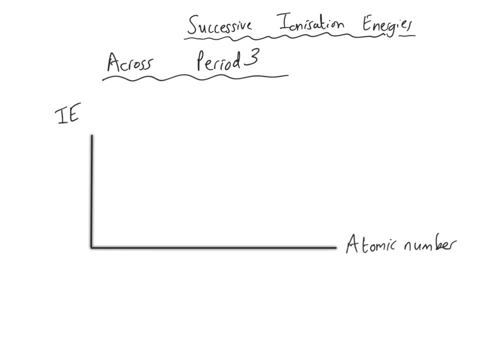 Now across period three. if we consider ionisation energies, the pattern is one of two, three, three. That's quite helpful to remember. And so, first up, if we just start, there's no numbers on this graph. This is just showing the general trend. It is an increase of two in there, or there's two in an increasing pattern. 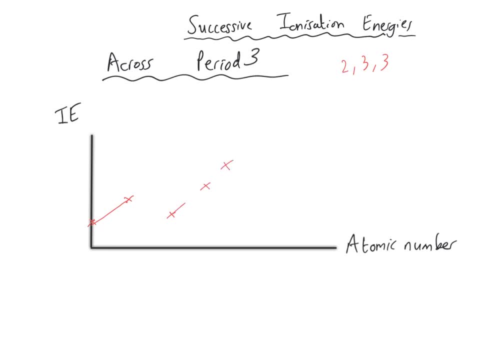 Then there is a dip and we've got three in an increasing pattern. And then there's another dip and we've got our last three elements of period, three in an increasing pattern. So overall ionisation energy increases across a period And the reason for those increases. 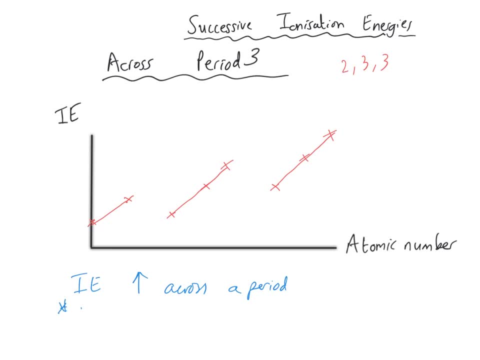 There's three reasons, or two reasons, and then an end result. And so, first up is that we get an increased nuclear charge for each element as you grow across the period, And secondly, the atomic radius decreases each time we move along one element in the periodic table. 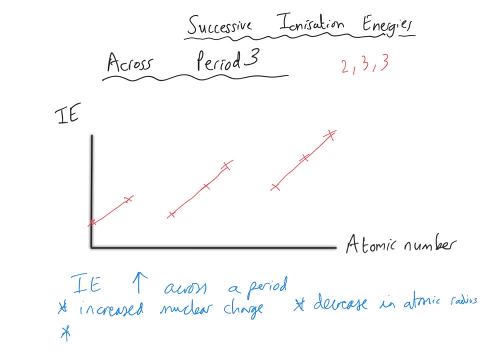 And then, thirdly, it's kind of a reason is that the electrons are in the same Energy level, and so that means that the shielding force that I mentioned before is the exact same for each of these elements as we go across the period, And so, overall, there is therefore a stronger attraction between the nucleus and the outer energy level electrons. 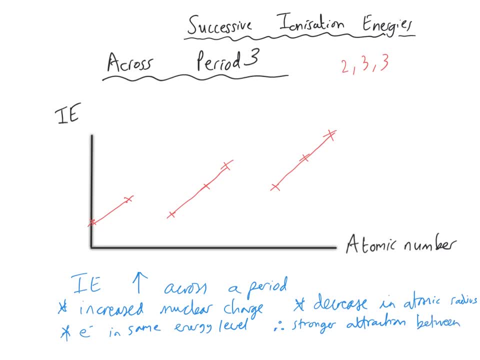 So this is greater attraction between the nucleus And the outer electrons, because not just any other electrons that are being removed, It's the outer electrons. There are, however, two dips in our pattern. The first step is easier to explain, And when you're asked to explain the cause of a dip, I think it's really useful to work out what the electron arrangement is for the different elements you're comparing. 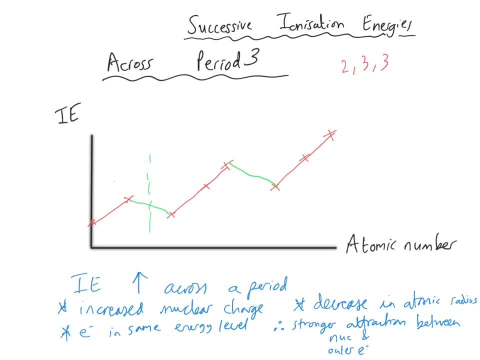 So we're in period three. So that means the second element in period three has got its own electron arrangement. The third element in period three has got its outer electron in the 3s2 subshell, Whereas for here, because we've got the third element in group three, it will be 3s2- 3p1, which means that the outer electron is being removed from a p subshell for this element on the right. 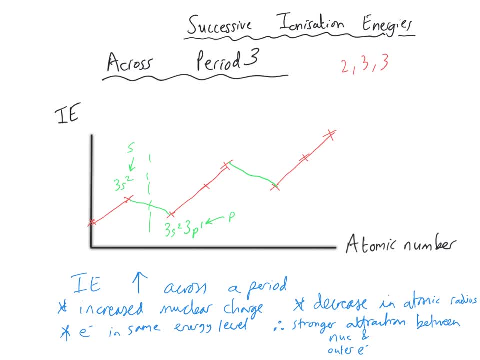 Whereas the outer electron is being removed from the s electron subshell for the elements on the left, And we know that p is a higher energy level, or higher energy, I should say, Then an s, And so therefore it is easier to remove. 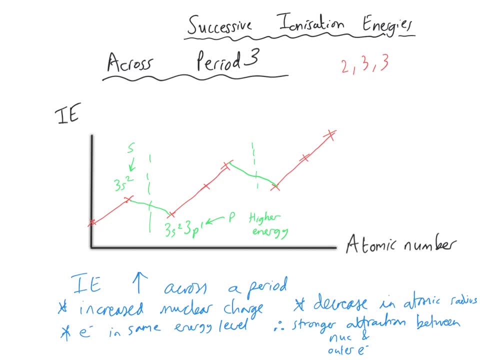 Over here. this dip in this region is a little bit harder to explain. But if we have a look again at the electrons, it's 3s2- 3p3 and this one is 3s2- 3p4.. And so what we're comparing is p3 to p4. 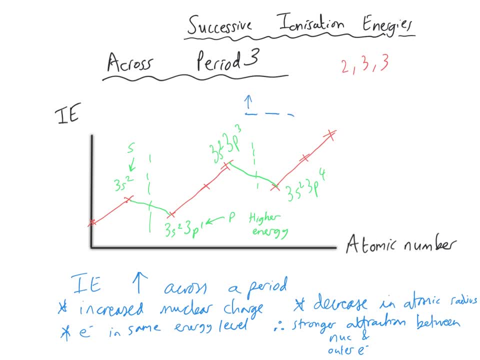 Now, if you remember that rule about the electrons occupying singly before doubly, what that means is in the orbitals. this element on here has got its own electron arrangement. This one here has got three single occupancy orbitals, Whereas down here- this 3p4, we've obviously only got room for three electrons to occupy singly. 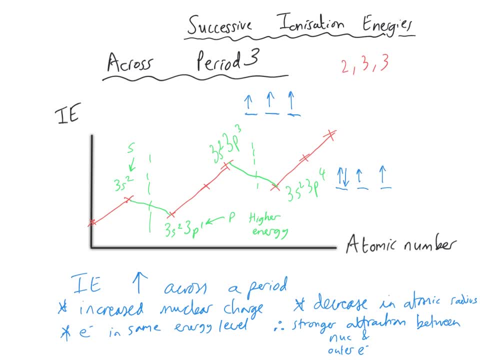 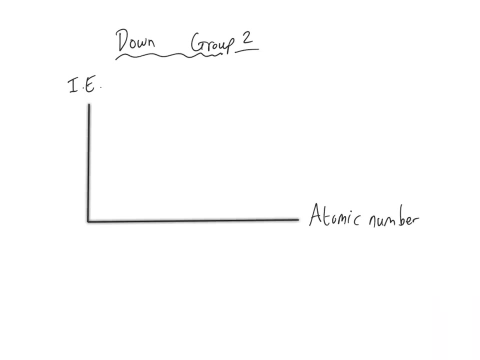 And so the fourth one has to pair up, And because of this thing called double occupancy, these electrons are easier to remove, And that's the reason for that second dip. as we move across period three, Group two is actually a little bit easier. 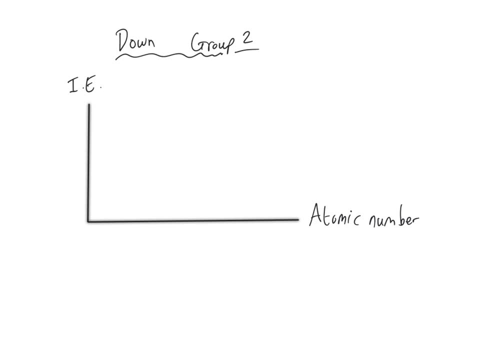 It just looks a little bit complicated because the first element that we have and then the second and then the third, that's a nice regular trend as atomic number increases, And then it stretches out. and it looks a little bit weird that it's stretching out like this. 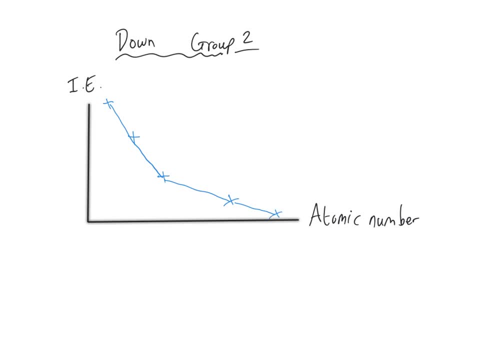 But actually the only reason for that is that we've moved into the D block, And so the number of electrons in a particular energy level increases from 2 to 8 to 18.. So the pattern isn't quite linear, But the general rule certainly is. 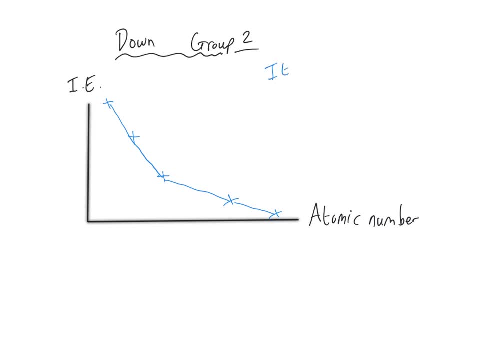 And that is that ionisation energy decreases down a group, And the reason for that decrease is really similar to the justification across period three. The atomic radius, though, is increasing, And as a result of that increase in atomic radius, there is weaker attraction between the nucleus and the atom. 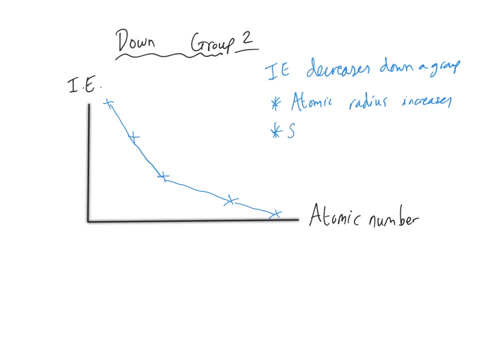 So there is more attraction between the nucleus and the outer electrons, But as well as that, shielding is also increasing. So that means that the electron shells are blocking the nucleus' attraction for the outer electrons And both of those factors end up with a weaker electrostatic attraction. 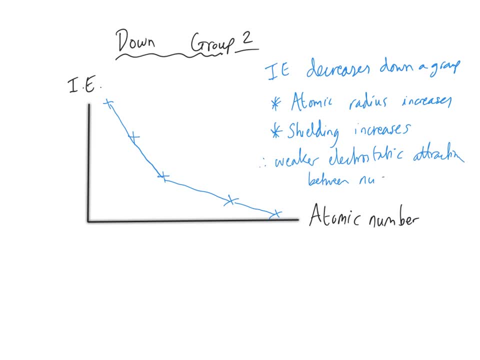 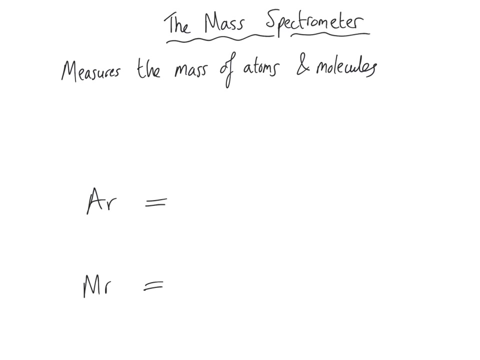 between the nucleus and the outer electron, Which is potentially being removed in the ionisation. We're going to move on now and have a look at the mass spectrometer, which is almost a separate section, but I've put it all in one video. 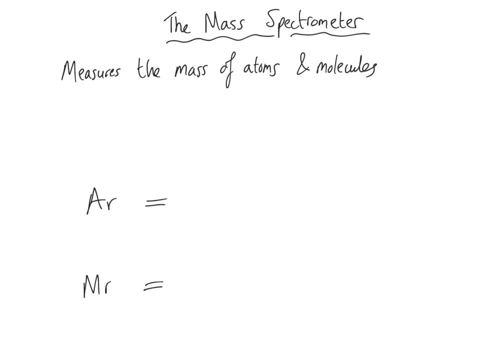 So a mass spectrometer is a machine and it's a machine for measuring because it's got the word meter or part of the word meter at the end, And that's a clue that it's measuring something, And what it's measuring is the mass of a particular atom or a molecule. 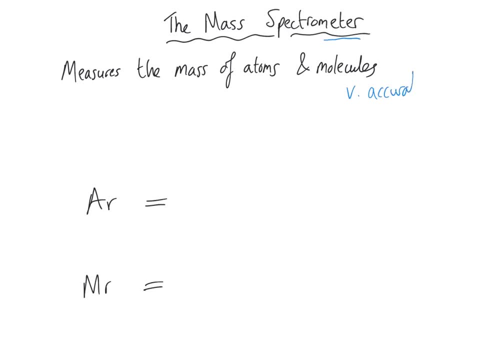 And a mass spectrometer is a machine for measuring. So a mass spectrometer is very, very, very accurate, And so it gives us a very precise relative atomic mass. And so the first thing that it can measure is it can measure the relative atomic mass. 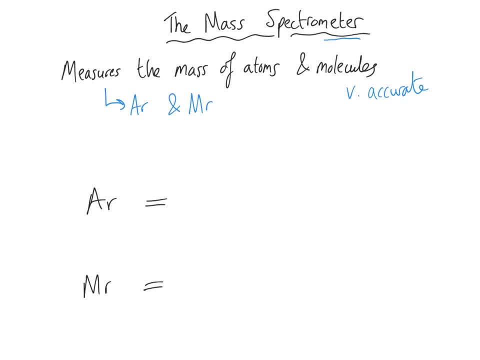 and it can measure the relative molecular mass for a particular substance, which is really useful. The second thing it can do is it can identify a particular element from its relative atomic mass value, because most elements have got a unique relative atomic mass And so if you know something's relative atomic mass, 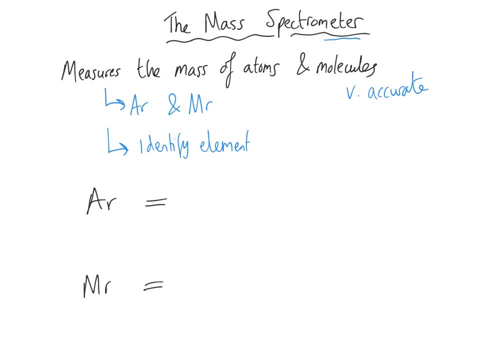 you can be pretty confident about its identity, although not always. I just want to take this opportunity to give you the definition for relative atomic mass and relative molecular mass. They're really, really simple. And what you do to calculate the relative atomic mass. 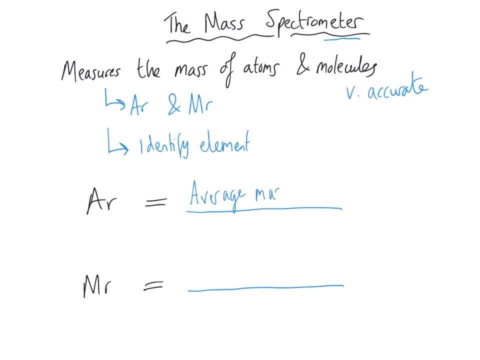 is you take the average mass of one particular atom and you compare it to the mass of a twelfth of a carbon-12 atom. So it's a twelfth of the mass of a carbon-12 atom, And then the relative molecular mass is very, very similar. 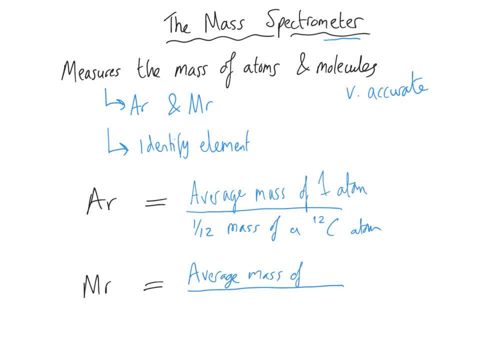 only. instead of it being the average mass of an atom, it's the average mass of one molecule, But we still compare it to the exact same thing. We compare it to a twelfth of the mass of a carbon-12 atom, And we use carbon-12. 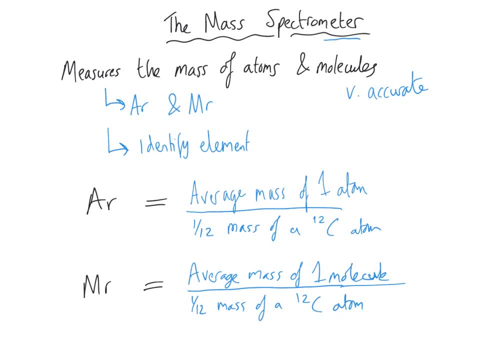 because it is pretty high isotopic purity. So it's about 99% of all carbon is carbon-12. And so we can be quite confident in our comparison, whereas other isotopes have got far more mixed proportions on there. So it's really important to know that we're comparing it to a carbon-12 atom. 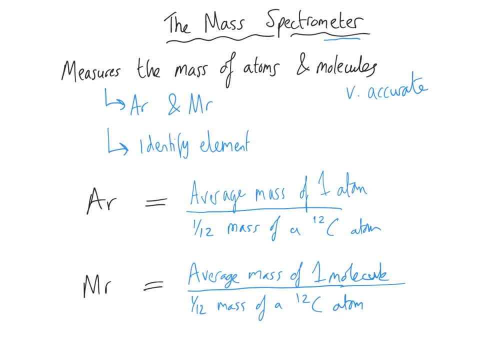 And because carbon-12 has got a mass of 12, what we're doing is we're comparing it to a twelfth of the mass of one of those atoms, because that allows us to get out. So that's our value of one if we take a twelfth of the mass of something that's got a mass of 12.. 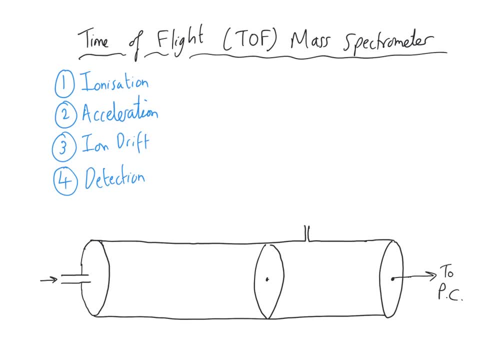 Now, what happens in the mass spectrometer? It depends on the mass spectrometer that you're looking at. What you need to know for your A-level course is a time-of-flight mass spectrometer which has got four main steps, And the first step is ionisation. 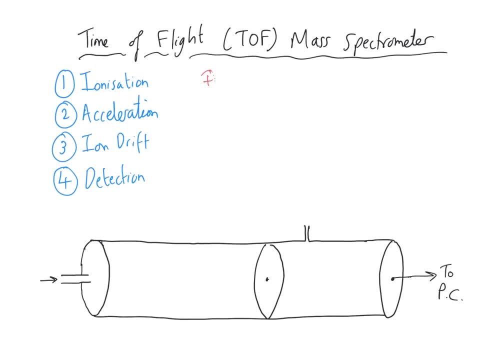 And, unsurprisingly, in that step we make ions And we need to know that we make positive ions in there, In that step, And I've got a pretty crude sketch of the mass spectrometer but the sample's injected here and ionisation happens in this stage on here. 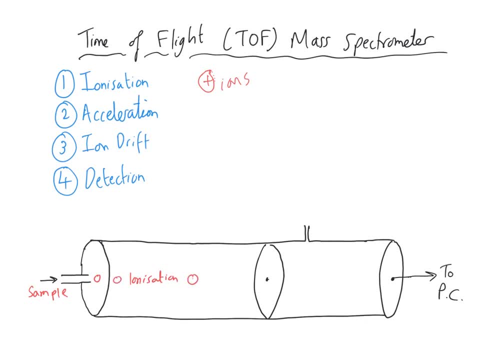 So here's our sample and here's our sample. And then it gets ionised so it becomes positively charged. Then the ions that are produced all accelerate across the gap. We've got a negatively charged plate over here. so obviously positive things and negative things. 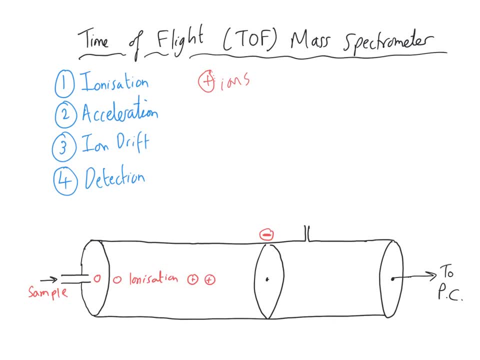 are attracted towards each other And this plate over here is fixed so it can't move. So these ions will drift across the gap on here. So that's what happens in here: We get acceleration because the ions gain kinetic energy And they all gain the same kinetic energy. 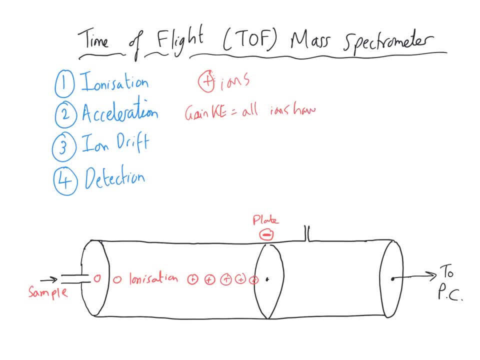 So all ions have the same kinetic energy, And what that means- because they've all got the same kinetic energy- is that the ions that are lighter will travel faster, Because if you push two things, and one's light and one's heavy, 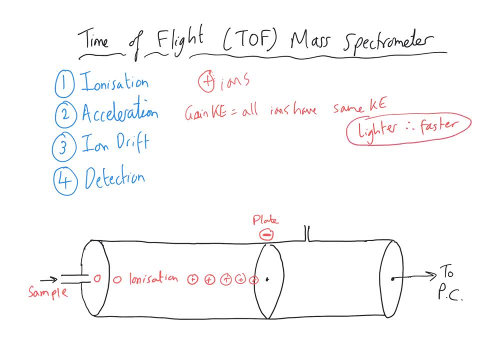 the lighter one will move faster. And so stage three, which is where the ions move along the tube. the lighter ones are going to move along the tube with a greater velocity When they get to the negatively charged plate. here there's actually a gap in that plate. 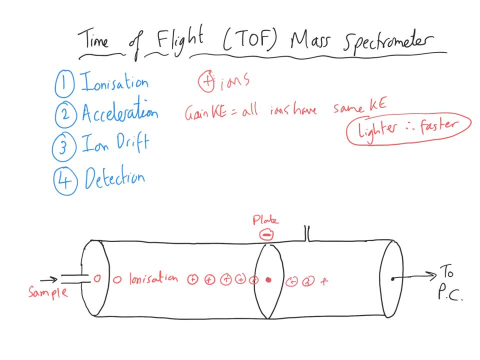 that allows the positive ions to pass through And that kind of focuses the beams that drift along here. And then the final step in the mass spectrometer is the ions hit a detector on here And, as I said, the lightest ones arrive first. 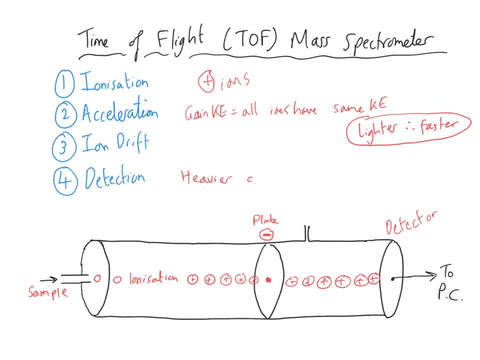 and the heavier arrive last, And then the detector sends a reading to a PC which gives you your display for your mass spectrum. And what I should say to finish off: this little side tube here, this is to a vacuum pump on here And what that does is that sucks all of the air out of the tube. 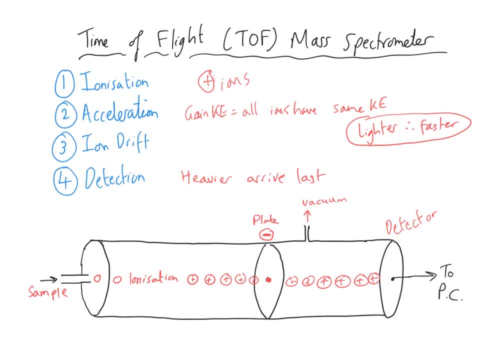 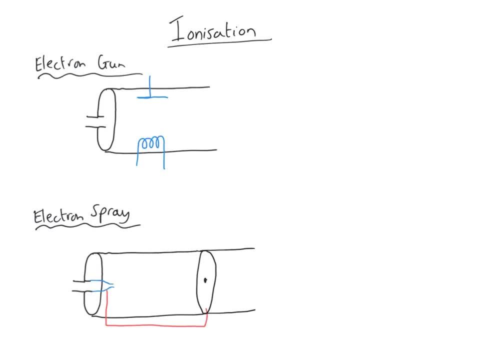 and that prevents our ions from colliding with air and being deflected off the path and never hitting the detector. Just want to have a look in a bit more detail about what happens in ionisation. There are two types of ionisation And you need to be careful when you're answering exam questions. 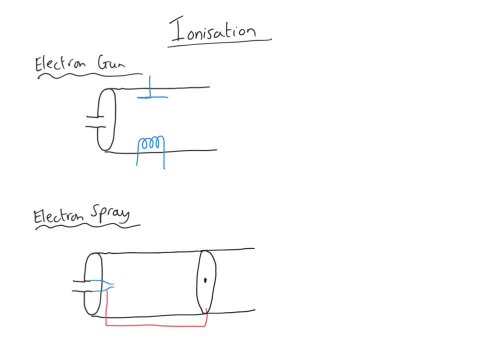 paying attention to which type of ionisation they are asking you about. There is the ionisation caused by an electron gun, which is what was on the old course And so that you'll find more past paper questions about the electron gun method And what happens in the electron gun. 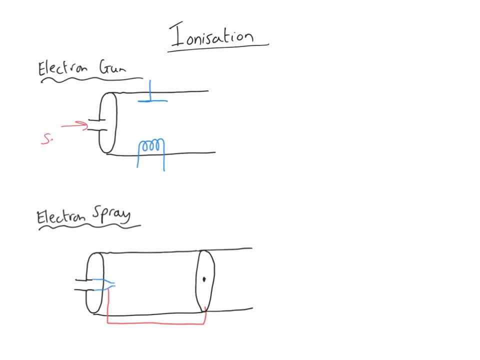 If you remember, the sample has been injected over here And we've got no charge. no charge, And what happens here is what We've got: a filament of wire that is very, very hot And that is a source of electrons. this hot filament. 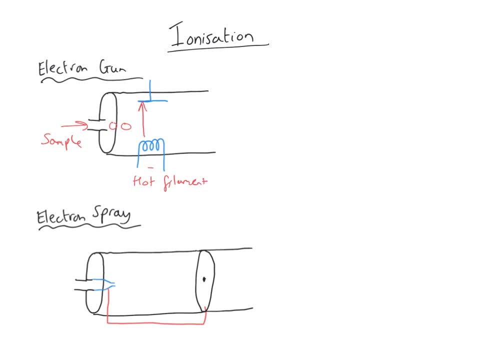 And what happens is the electrons get fired across this gap over here towards this positively charged plate, And the sample that's moving through the flight tube gets hit by those electrons and more electrons get knocked off. So we've got our gaseous sample. 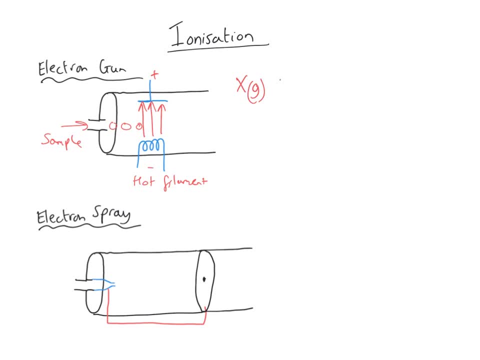 because the sample that passes through the tube has got to be a gas And we hit it with an electron and that knocks another electron off. So we end up with a gaseous ion And we end up with two electrons, because we had one that was from the gun. 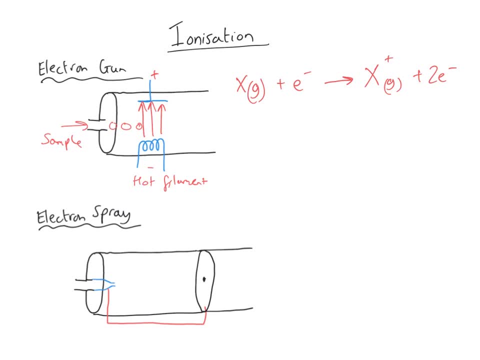 and another one that has been knocked off. Alternatively, you can write this equation slightly more simply by removing the electron from the electron gun and just only writing down in the equation the electron that was knocked off from the sample. Then the second technique is new to the course a few years ago. 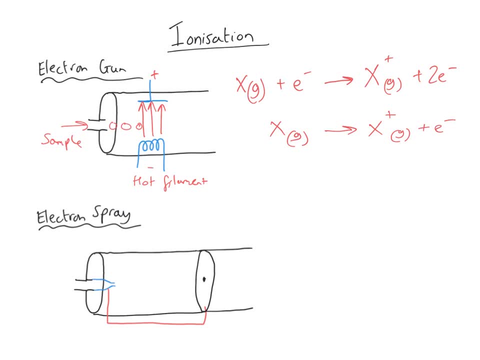 So you've got fewer questions about this electron spray technique, And this also happens in the early part of the flight tube. And what you've got here is you've got a needle And so the sample gets injected, But what happens is it gets dissolved in a volatile solvent. 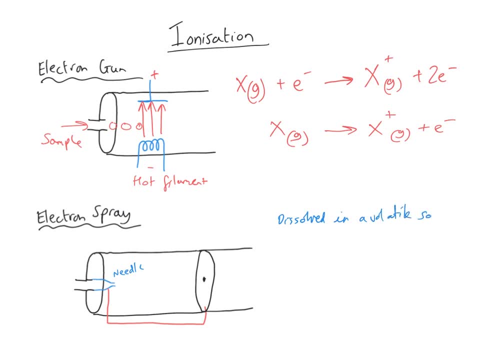 And then it's forced through a needle, And as it's forced through a needle, a high voltage is applied, And what that causes to happen is the sample gains a proton, And so what we have here is we've got our sample, which I'm just going to write as X again. 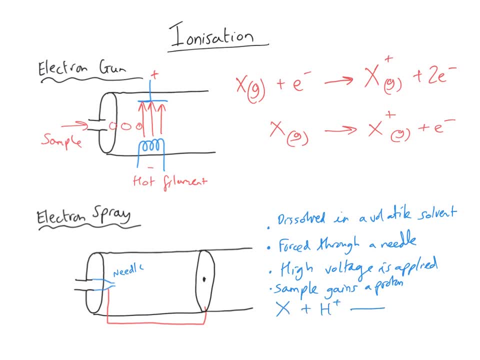 And it gains a proton. And so what happens is we end up with a slightly weird looking thing, which is our sample, with a proton joined to it, an H plus joined to it, So it's slightly heavier than before, which is worth noting. in a minute, 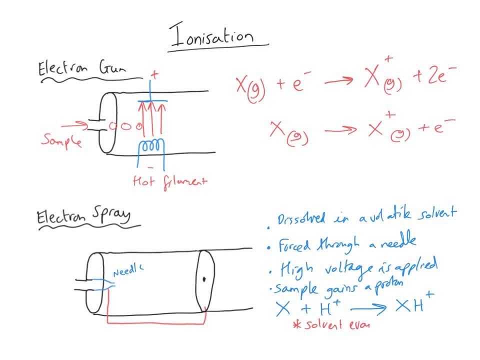 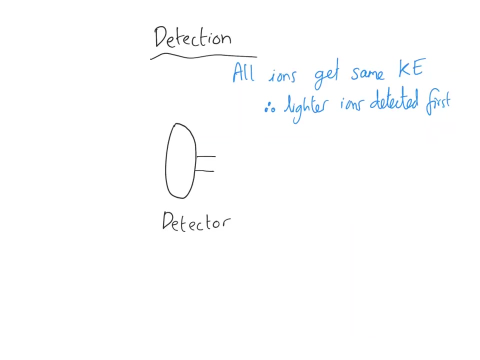 And then, last of all, the solvent evaporates to form gaseous Positive ions, to form XH plus as a gas, And so the ions have drifted through the tube and they come towards the detector over here. Now remember, all ions get the same kinetic energy. 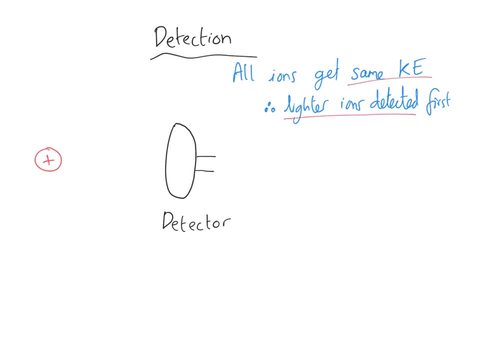 which means the lighter ions get detected first They've got a shorter time of flight. That's where the phrase time of flight mass spectrometer comes in. They're detected first, They have got a shorter time of flight, And so the ions are drifting towards the detector. 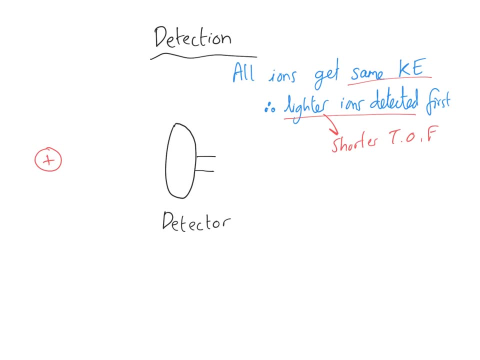 They hit the detector. There's a positive ion hitting the detector, And so what happens is the positive ions pick up electrons from the detector and that causes a current to flow. Now if we've got a really abundant particular ion, a greater number of electrons will move off the detector. 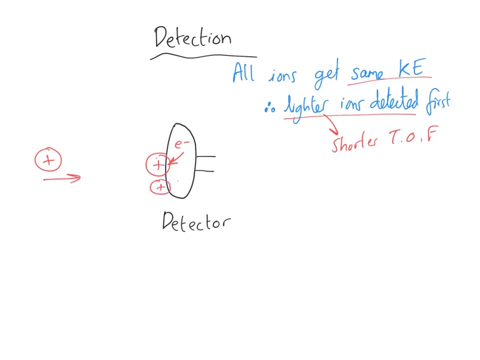 and move away. So if we've got a really abundant particular ion, a greater number of electrons will move off the detector and move away And move towards the ions And so we'll get a greater current. And so our conclusion on here is: if we get a larger current, 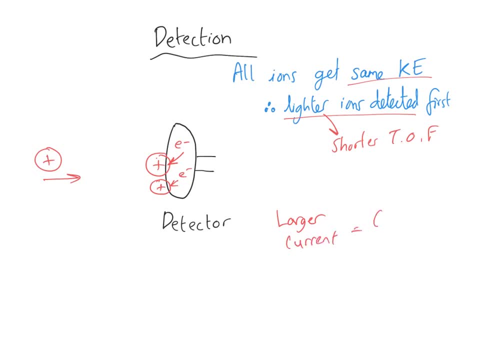 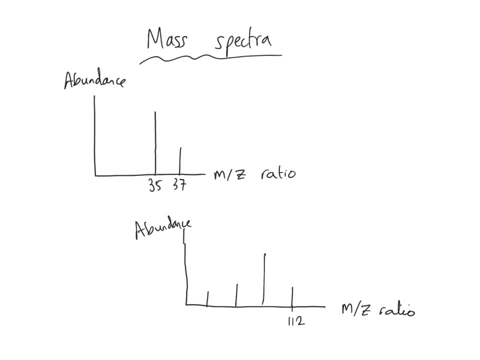 we've got a particular ion or substance that has got a greater abundance. That means there's more of it in our sample. So what does a mass spectrum actually look like? So we've got two spectra on this slide on here. The first one is showing us one particular 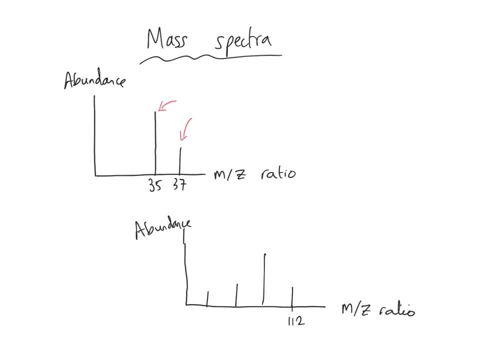 quality of mass spectra, which is where you have isotopes. you get a peak for each isotope that is present, And so these are isotopes of chlorine, And so we have some chlorine which has got a mass of 35. And we've got other chlorine that's got a mass of 37.. 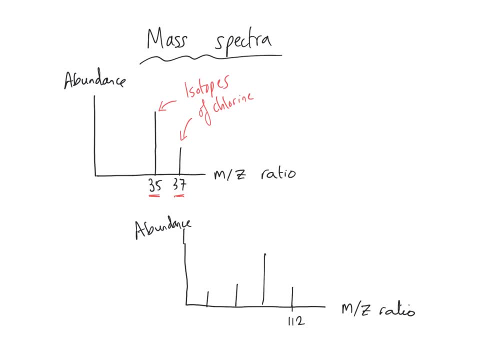 And that's coming up on this x-axis as a MZ ratio And that's referred to as a mass to charge ratio. And that mass to charge ratio is really quite simply calculated because normally if one electron is removed or one proton is gained, 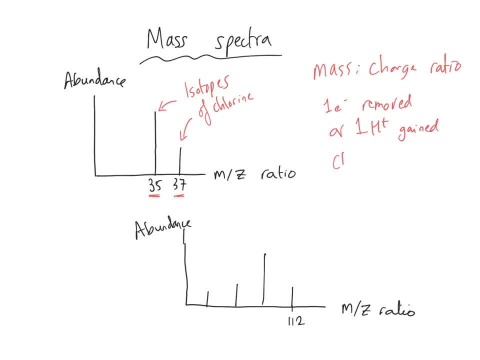 that means that the charge is going to be one plus, And so if the charge is one plus, that means that Z the charge is one, And so that means that MZ is effectively the M mass if the charge is one. 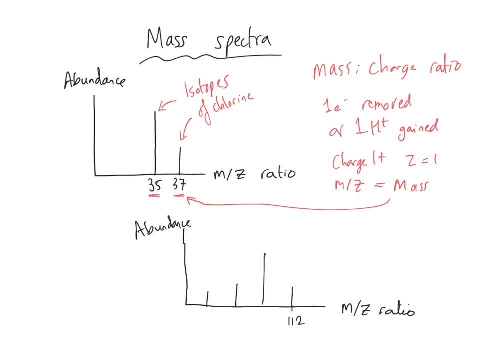 And so what that means to go back over here is that we've got chlorine with a mass of 37 and chlorine with a mass of 31.. Now, I've tried to draw these to scale, because what we can learn on here is we can track across the abundance. 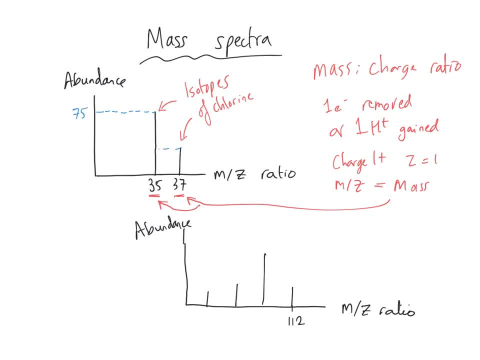 and we can find out that 75% of all of our chlorine 35 and then 25% of all of our chlorine is chlorine 37. The slightly heavier isotope of chlorine Abundances might be a percentage or they might not. 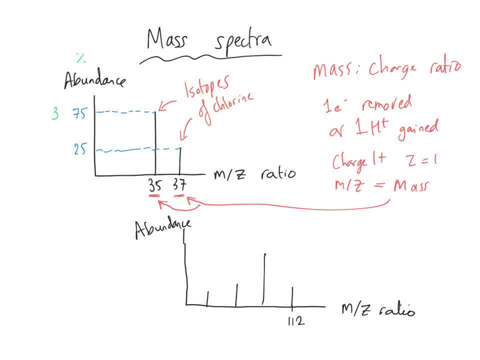 It might just be a comparison, because 75 to 25 could just be 3 to 1 as a proportion on there. It doesn't have to be a percentage. The second useful thing about mass spectra is shown on this second spectrum down at the bottom. 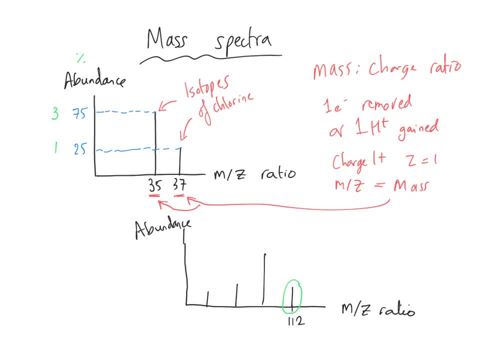 And that involves the peak, that is the furthest to the right In a mass spectrum, which is the heaviest peak. The heaviest peak, the one with the greatest MZ ratio, is always the molecular ion peak, And so what that means is you've got the whole molecule. 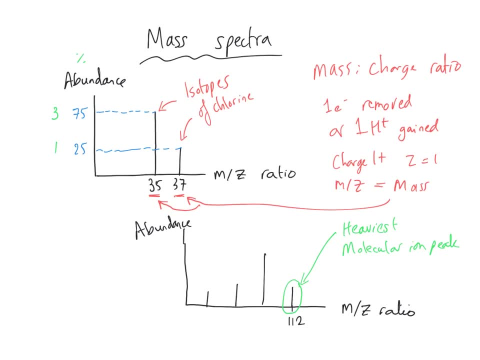 that has either had one electron knocked off it or it has gained one proton, And so this molecular ion peak is absolutely vital, because it tells us what the MR is for a particular substance. So for here, for my made-up sample, my made-up spectrum. 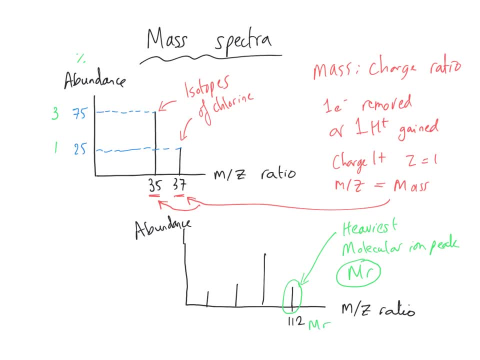 we've got an MR of 112 from this substance And that can help us to identify what that substance is. Another little quality of mass spectra is we have peaks, not just the molecular ion peak, but we also have slightly lower MZ values. 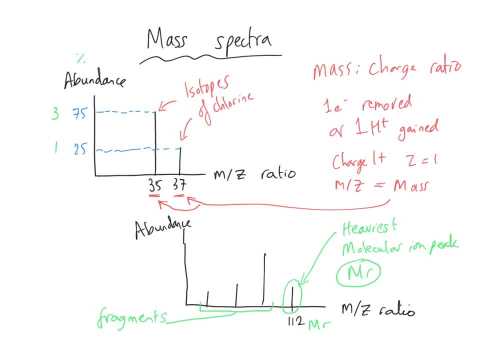 And this comes from something called fragmentation, And these are peaks for particular fragments of the molecule And that's because it's particularly common in the electron gun ionisation When an electron gets removed from a covalent bond that's holding two atoms together. 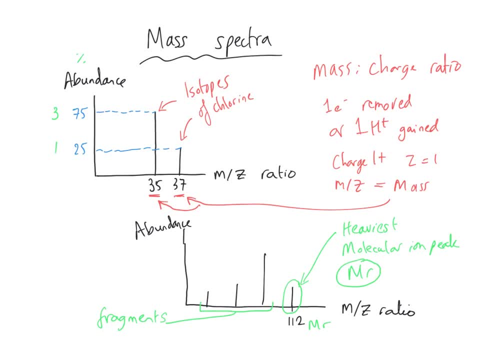 we've only got one electron holding the atoms together And that isn't really enough attractive force to hold those two atoms together. So they fall apart into pieces And one of those pieces will be positively charged And it's that that gets detected in the mass spectrometer. 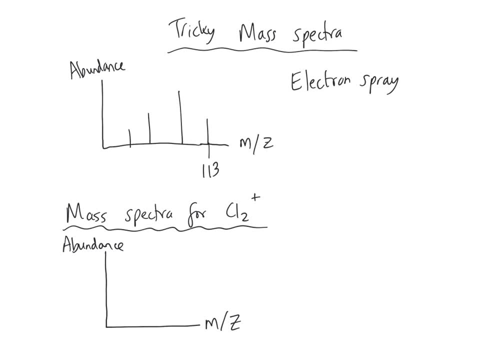 Just to look briefly at slightly more tricky mass spectra. the first one isn't really particularly tricky, It's just a notable difference from the previous mass spectrum on the previous page, And this one has been generated using the electron spray mass spectrometer, And so when you ionise using that, 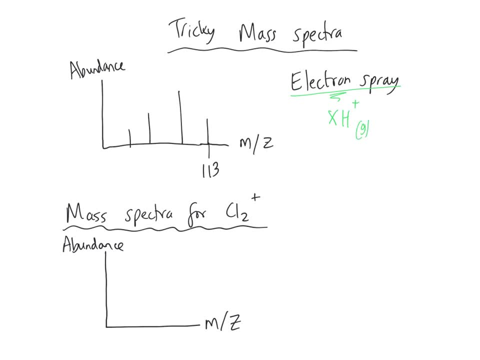 remember that what you detect is the gaseous sample that has gained a proton. So you're detecting something with an MZ value that is one higher than whatever the MR is. So this 113 over here, that is for the substance with an extra proton. 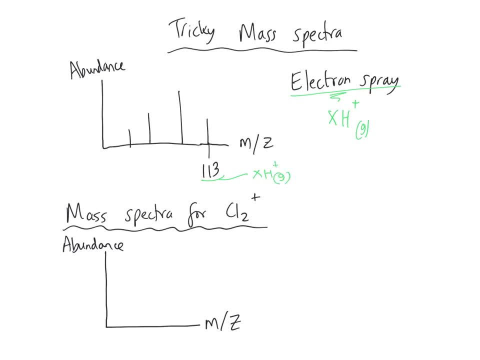 a hydrogen ion, And this hydrogen ion has got a mass of one. So that means that the MR of this substance is actually 113. take away one- Not complicated maths, but you might forget to do it, So you need to take away one from the MZ value. 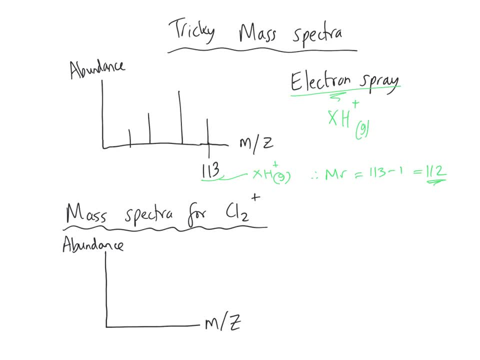 when you're working out what the relative molecular mass is for a sample if it's been ionised using electron spray. That's what I was saying when I mentioned about paying attention to what ionisation technique they mention in the question. And then, last of all, 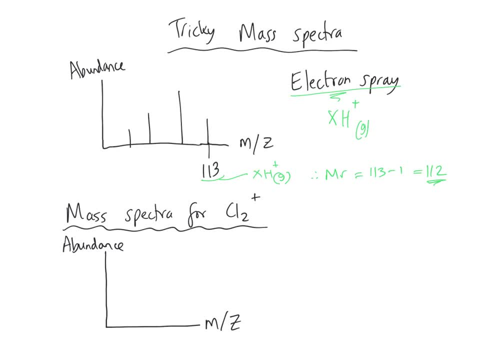 a tricky mass spectrum could be, for when we have a molecule of chlorine. Now, this is tricky because there's two atoms in Cl2, obviously. but they could. both could have different masses, So they both could be different. They might not be different, but they could be. 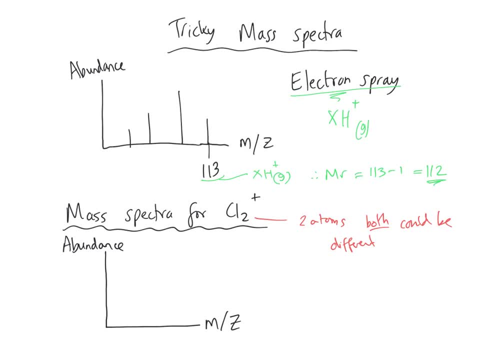 And so what we could have is: we could have. if we consider, say, chlorine atom A and chlorine atom B, chlorine A could have a relative atomic mass of 35. And so could chlorine B. Chlorine A could have a mass of 35. 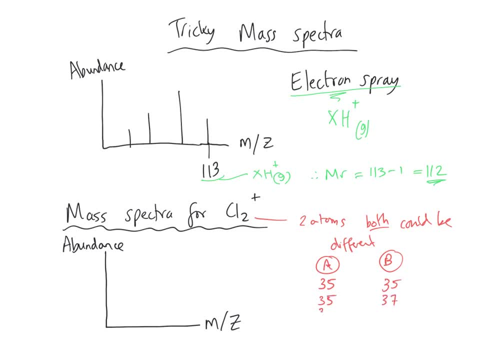 Chlorine B could be 37. Chlorine A, though, could have been 37, and chlorine B could have been 35. And then the last combination that's possible is 37 for both of them, And so what that means is that 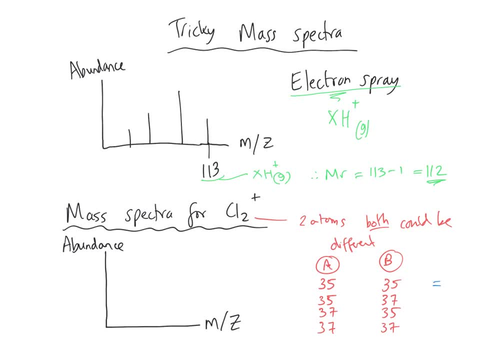 when we combine those two together, that has got a total mass of 70,, that's 72, that's 72 as well and that's 74. So the mass spectrum for chlorine will have three peaks: one at 70,, one at 72,. 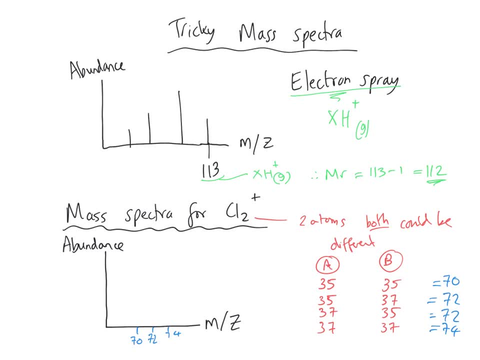 and one at 74. And they won't all necessarily be the same height. In fact they definitely won't all be the same height in this instance on here, And the reason for that is kind of statistics and in maths that three quarters of all of the chlorine 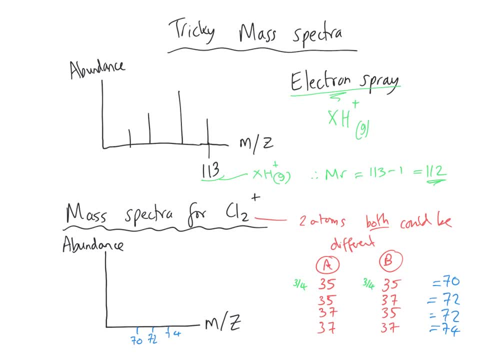 is chlorine 35. So that means there is a three out of four chance that this atom over here will be chlorine 35 and a three out of four chance that this one will be as well. So that means that there is a nine out of 16 chance. 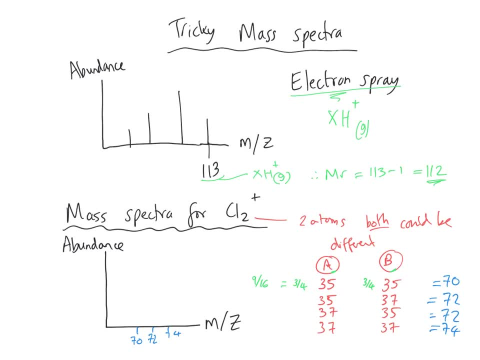 that they will both be in chlorine 35. The probability that the first chlorine atom is chlorine 35 is three out of four. If the second one is going to be the heavier chlorine 37 isotope, that is not so likely, And so there is a three out of 16 chance. 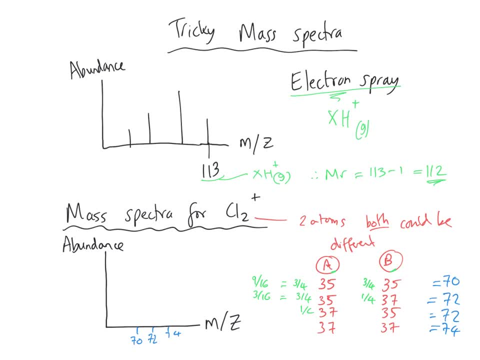 of this combination. The third combination is the exact same odds just the other way around, And so that's a three out of 16 chance on there, And then the last combination is actually only a one in 16 chance that we're going to get that. 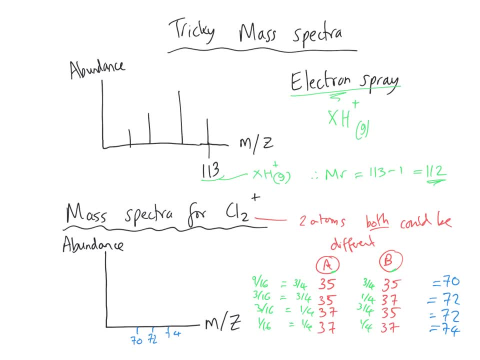 So if we were to draw these peaks, the chlorine 37, 37, so the one with an MZ of 74 would not be very high at all. Its abundance would be one or one out of 16, but I'm just going to call it one. 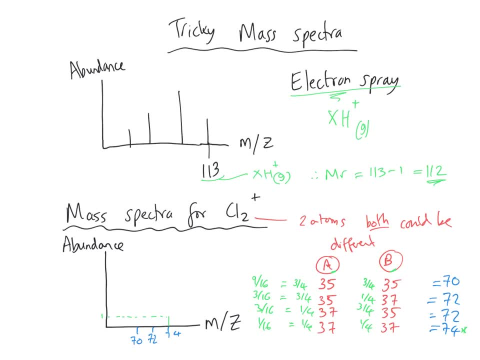 by taking the first digit in my fraction, The peak at chlorine 72, because we've got two that combine together, we've got a six out of 16 chance that chlorine will be chlorine 37.. 72, CL2 with 70.. And so that means that this abundance 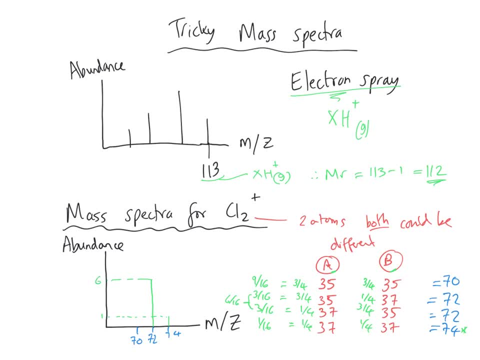 would be a size six. And then, last of all, the greatest probability, because it's nine out of 16. well, that tells us that it needs to go all the way up to here, to what would be nine for the abundance on here. So we would have three peaks. 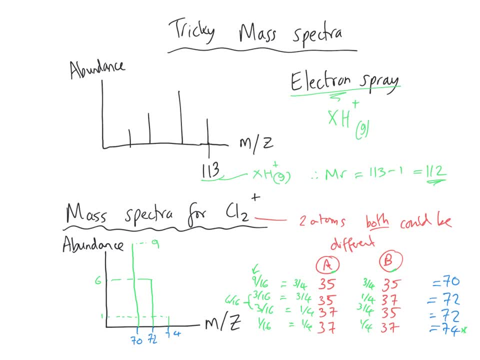 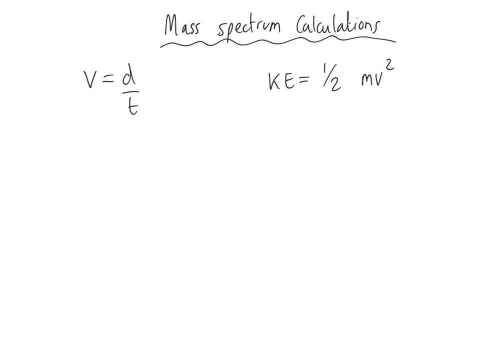 and the chlorine 70 would be the tallest peak of all, followed by chlorine 72, followed by chlorine 74. It would be in terms of their abundance. it would be a nine to six to one ratio. Let's have a look now at mass spectrum calculations. 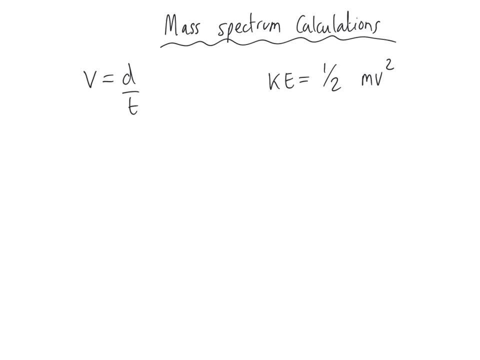 There's two equations that you need to be able to use, and you'll probably get given them in the exam, but it's worth getting familiar with them in case you don't get given them, And so the first one is the equation that you learnt at GCSE level. 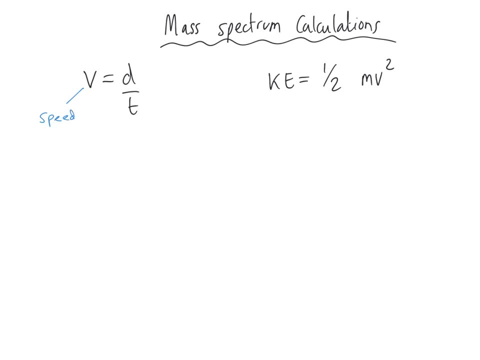 where we're looking at speed equals the distance divided by two times the time. Now we use the symbol V because what we're really talking about is we're talking about the velocity that these ions are moving through the mass spectrometer, and that is in metres per second. 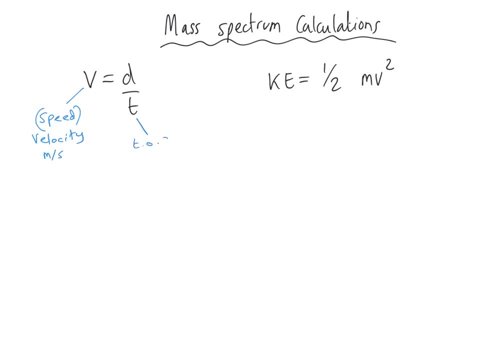 T is the time of flight, and that is in seconds, and D is the distance, that's really the length of the time of flight. mass spectrometer, and that is in metres. Ke is the kinetic energy, and that's in joules. Remember that is the same. 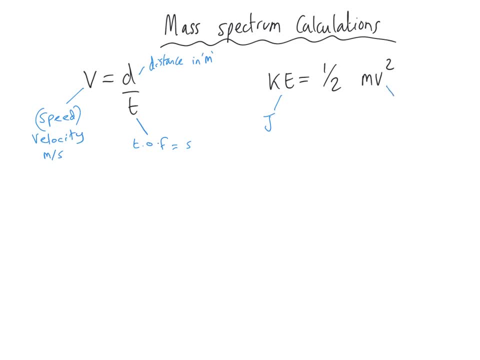 for all of the ions that can be really important. V- this is once again the velocity of the ion in metres per second, but then we're going to square it. And then, last of all, this M: this is the mass of one ion. 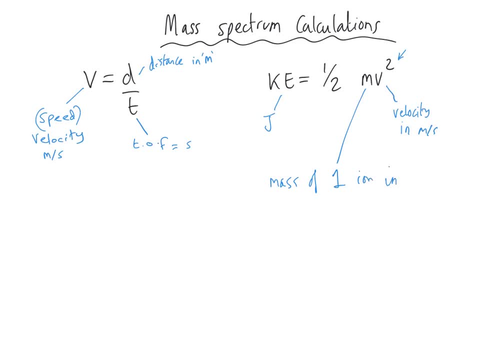 And, slightly confusingly, it's the mass of one ion in kilograms. So what that means is, if we know the relative atomic mass, what that tells us is the mass in grams of one mole, And so what we then need to do is we need to divide that. 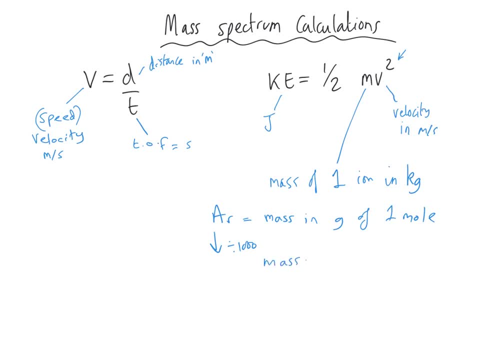 by a thousand, because that will give us the mass in kg of one mole. And then we need to divide by Avogadro's number, 6.022 times 10 to the 23, because that will then give us the mass in kilograms of one atom. 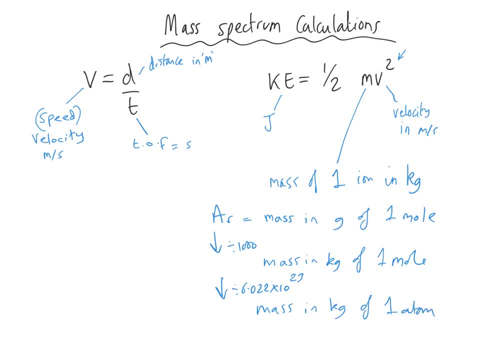 Because in one mole there are 6.022 times 10 to the 23 atoms, and so we divide by that number to find the mass in kilograms of one atom. It's quite complicated to keep saying that number again and again and again. So Avogadro's number: 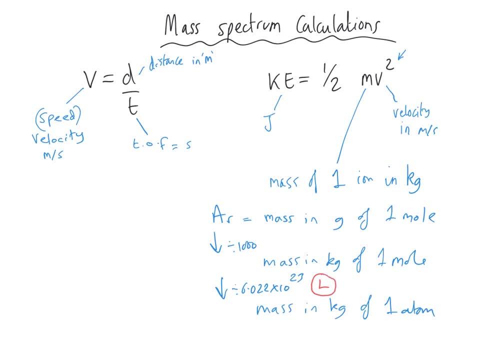 has got the letter L, capital L, if we wanted to use that in calculations, Just by the by, because we're talking about ions, even though it is an ion, that means it's lost an electron, Because the mass of an electron is practically zero. 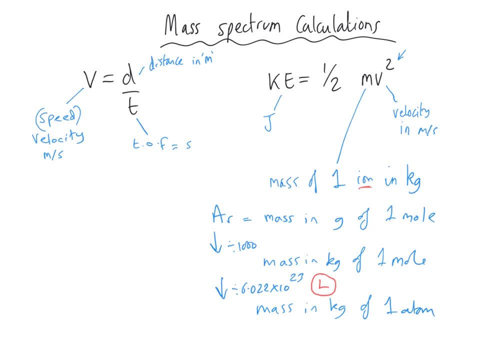 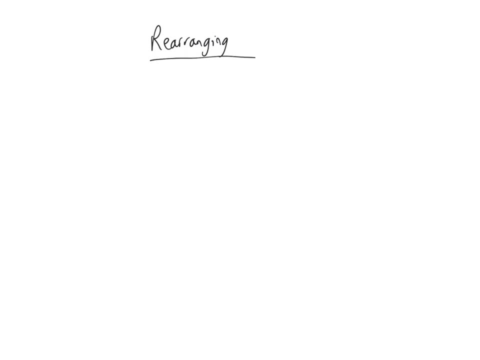 that means that we can assume that the mass of an atom is the same as the mass of the ion that it would form. Just a quick note about rearranging these equations. So speed equals distance divided by time. So that means we've got distance divided by time. 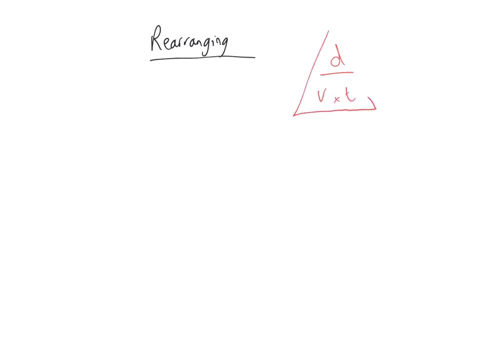 and we've got V on there And so that is a formula triangle here. So you'll be familiar with from GCSE level. And then kinetic energy is half mv squared. Some people like to just remember the rearranged formula because they don't like. 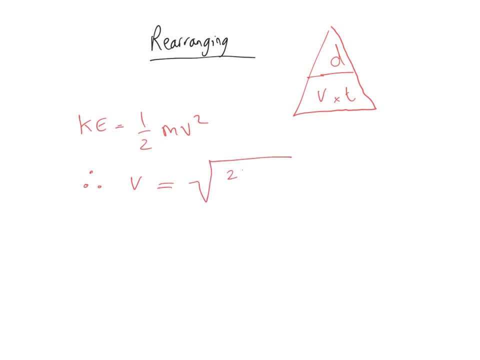 rearranging things. And so that means the velocity is two times by the kinetic energy divided by the mass of one ion in kilograms. Now remember, whenever you do one of these calculations, particularly if you're working out time of flight to do what's called. 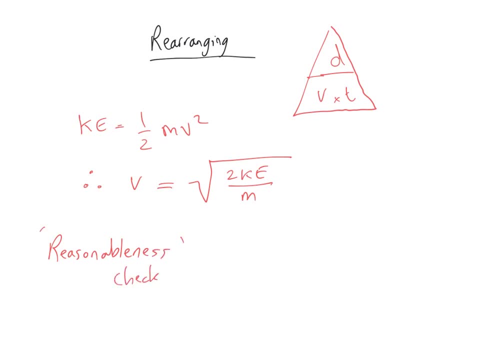 a reasonableness check, And what that means is: does my time seem feasible? Because if I've done a calculation and I've been given the time of flight for one substance and then I'm calculating the time of flight for something else that is heavier, 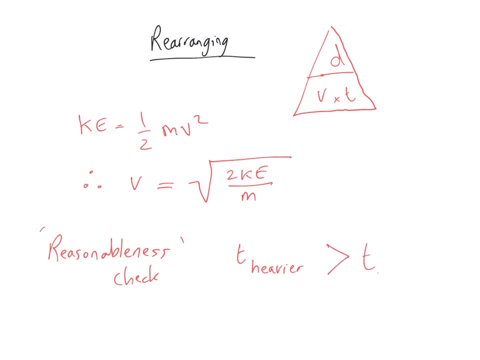 then I need to be aware that the time of flight for an ion that is heavier should be greater than the time of flight for something that is lighter. It might not be very, very different, but it should be heavier, And the numbers are often. 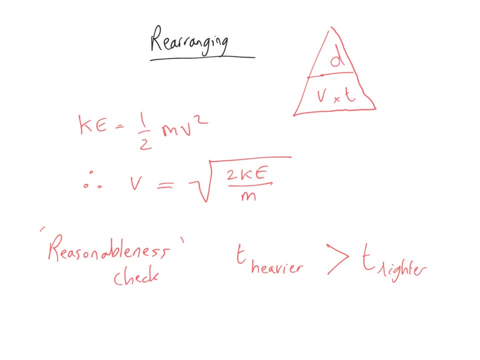 really quite small. It doesn't take very long for the ions to go through this tube, So just be aware that the answer is likely to be in standard form and very, very small. The last thing about calculations in the mass spectrometer that I wanted to show you. 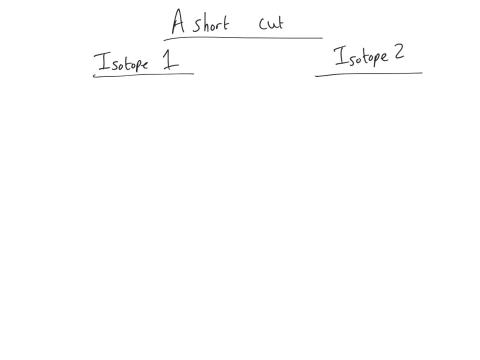 is a shortcut, And that shortcut can be used by making several kind of connections between these two equations and between what happens for one isotope and it being the same when we're considering another isotope. The first thing that we need to do is we need to consider: 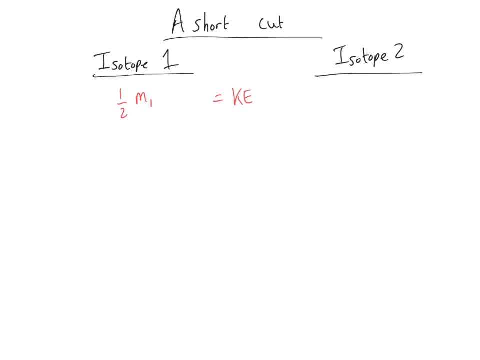 the kinetic energy of each of these isotopes, And the kinetic energy is half mv squared for each of them. I'm just using little subscripts, one and two, to show the masses of the two different isotopes and masses and the velocities of the two different isotopes. 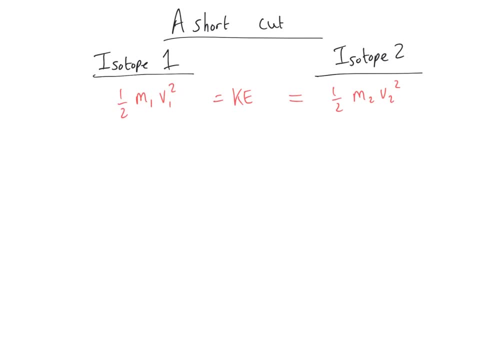 on there. So kinetic energy is mv squared for both of them. Now, since it is the same for both, we can merge those together and no longer have the kinetic energy in the middle. Half mv squared for the first isotope is going to be. 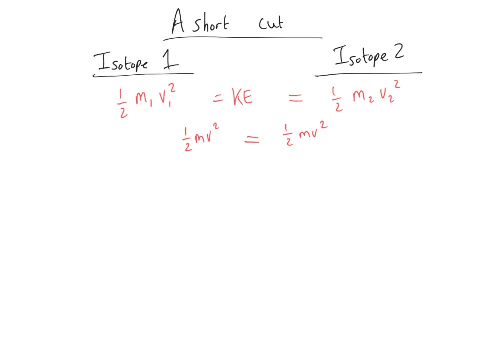 half mv squared for the second isotope, Then I'm going to make it slightly more complicated before making it a lot easier. So if we substitute in that calculation for how you work out the mass of one atom or one ion, I should say: 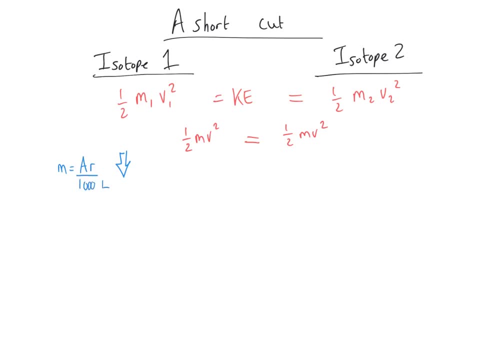 by taking the relative atomic mass and dividing it by 1,000 and then dividing it by Avogadro's number, what we're going to end up with is we're going to end up with half times by the relative atomic mass of the first isotope. 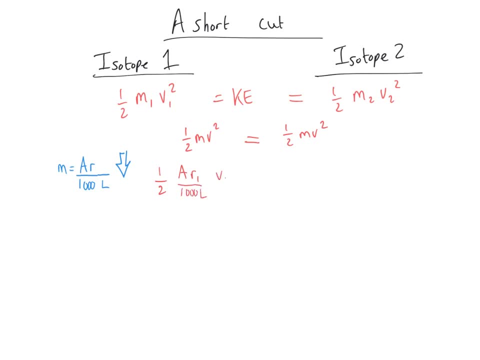 divided by 1,000 times by Avogadro's number, multiplied by the velocity of that isotope squared, is equal to a half times by the relative atomic mass of the second isotope divided by 1,000 times by Avogadro's number. 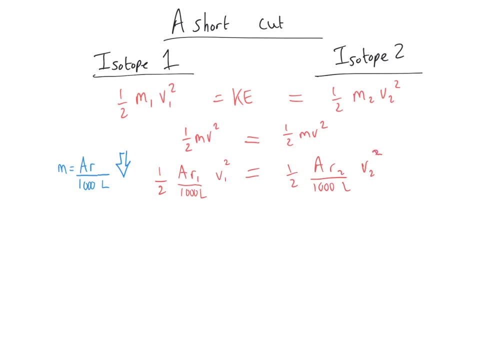 and then the velocity of that ion squared. And then we need to substitute in one last time for v. speed is distance divided by time. So when we substitute that in we've got half times by the relative atomic mass of the first isotope. 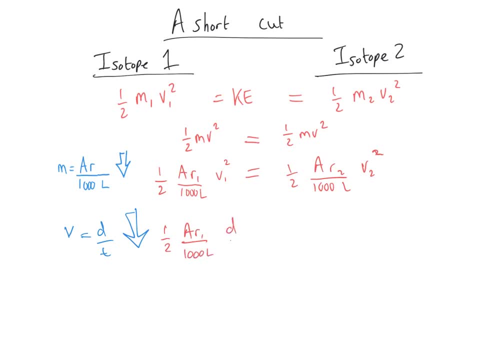 divided by 1,000, L multiplied by the distance, and then the time of flight is on the bottom over there, That T1 is the time of flight for ion number one, And we do the exact same thing for the second isotope And we're left with an equation. 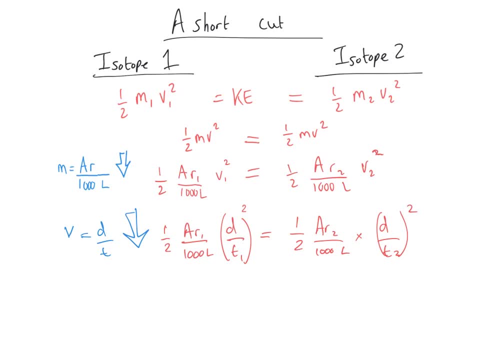 that looks really complicated, but it's about to get really simple, because whenever you've got something on one side of an equation and you've got it on the other, that is the same on both sides. we can get rid of it, So there is no point. 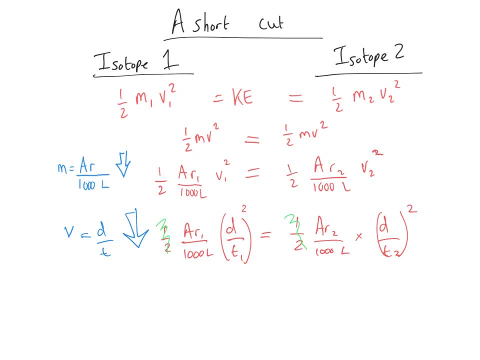 multiplying this number by a half on both sides, So we can get rid of the halves, because that's present on both sides. We can get rid of the thousand on both sides, because that's the same on both times, And then we can get rid of. 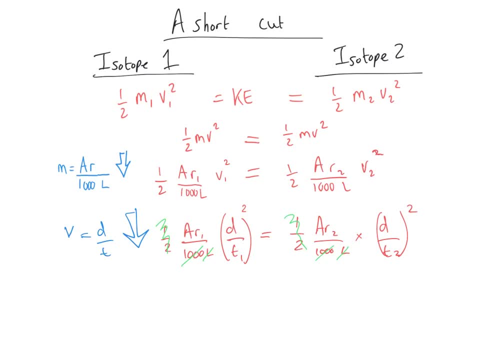 Avogadro's number, because that is a constant, one of the fundamental constants in chemistry. We can get rid of that from both sides. We can also get rid of the d from both sides, because both of them, both of the ions, will be passing through. 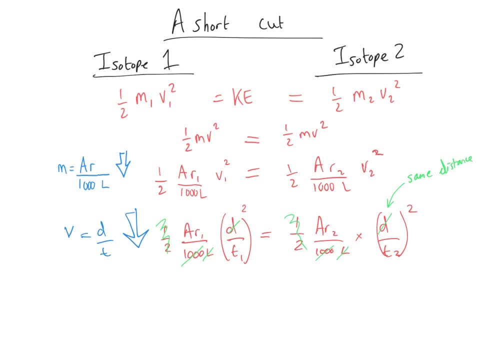 the same tube, and so they'll be travelling the same distance, And so d will be a constant value as well. So once all those numbers have been taken away, we've got the relative atomic mass of the first ion divided by its time of flight. 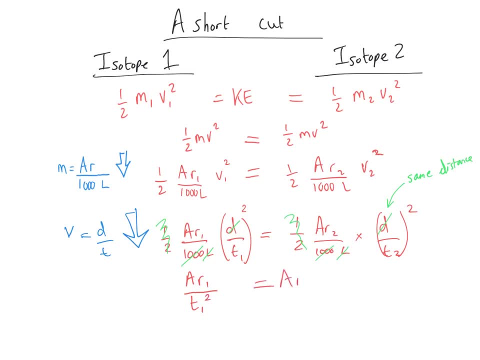 squared will be equal to the relative atomic mass of the second ion divided by its time of flight squared. And so that little box, there is a really nice kind of shortcut memory aid, whatever you want to call it, a way to help you work fast. 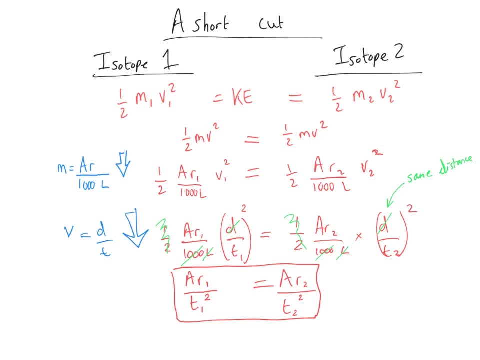 particularly if you're calculating the time of flight for a particular isotope- And that can rearrange, by the way, if you like it in a rearranged form, because you don't want to remember something that is hard to rearrange- then the time of flight. 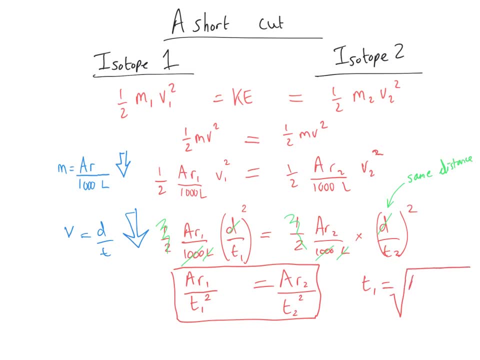 of the first isotope is the square root of the atomic number of the first isotope times by the time of flight of the second isotope, squared divided by the atomic number of the second isotope on there. So that's another form for that same equation. 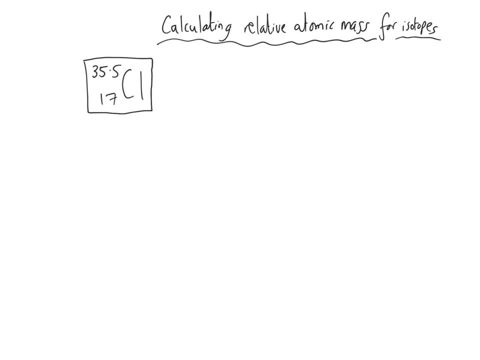 Let's finish this video by considering a couple of last few things about isotopes. So the first thing to consider is something that you will have known for some time, which is that chlorine has a relative atomic mass that is not a whole number, And this is an average. 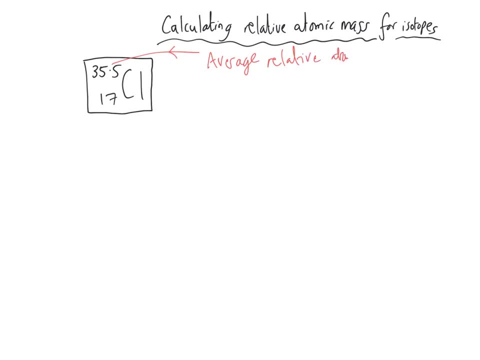 relative atomic mass. And what that means is if we had 100 chlorine atoms and we put them all in a box and we found out how heavy they all were together- the total mass of those 100 atoms- and then we divided it by 100. 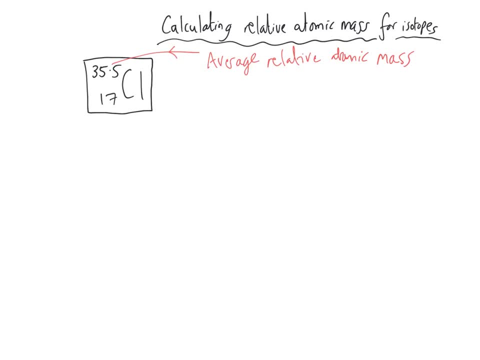 to get our average, the number that we would have is 35.5.. But you would not find a single chlorine atom that had a mass of 35.5.. What you would find, as I mentioned on a previous page, is that you'd find chlorine. 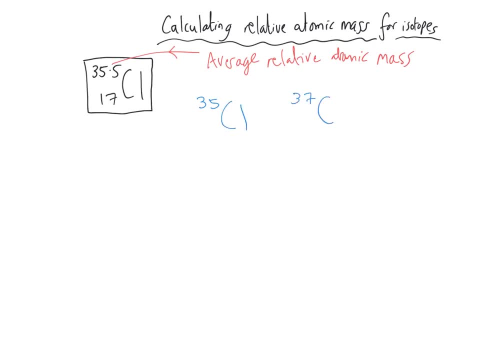 that had a mass of 35, and chlorine that had a mass of 37.. 17.5.. That's the number of protons for each of them, by the way, And the abundance of those, as I showed you on the mass spectrometer page. 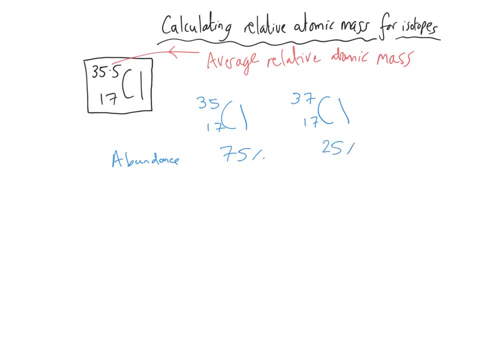 is 75% of this one and 25% of this one, And so what that means is: how do we calculate our average? Well, the relative atomic mass is found by taking the abundance of one isotope multiplied by the relative atomic mass. 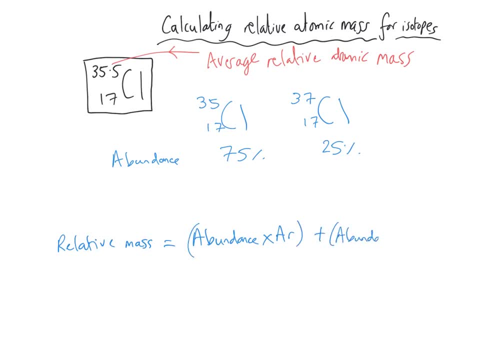 then we add it to the abundance of the second isotope times by that relative atomic mass, and then we divide it all by the total abundance. And if there's more than two isotopes, we just kind of keep going on and on and on for however many. 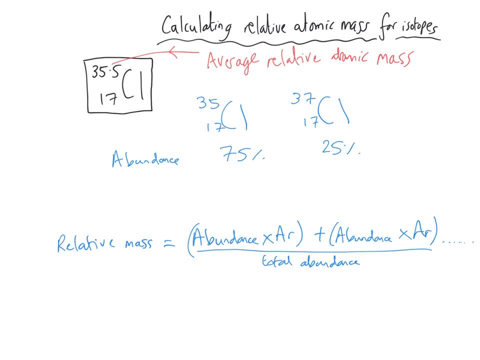 that there might be three, four. I can't imagine there'd be more than three in an exam question. that'd be a bit mean. And so what that means is that we can do a sum where the average mass for chlorine is 75,. 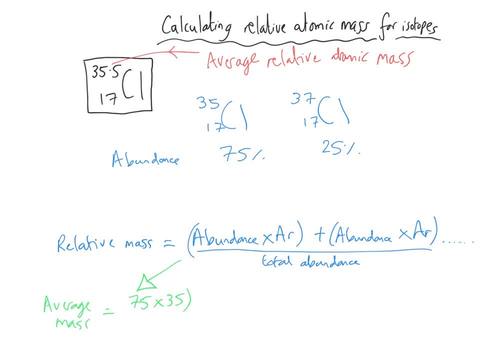 multiplied by 35,, added to 25 times by 37, and then all divided by 100 over there, And that gets us our 35.5 as our answer. Now, if the abundances aren't given as percentages, we do the same thing. 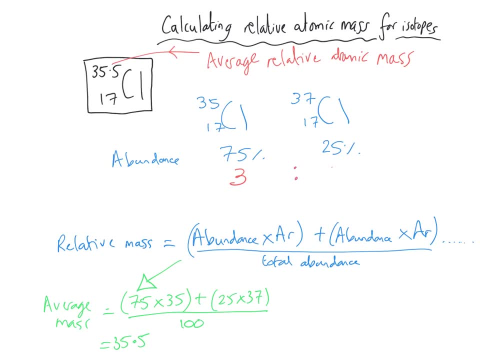 So 75 to 25,, as I said before, is a three to one ratio, a three to one proportion, And so the total abundance doesn't always have to be 100%, like it is here. The total abundance could be four. 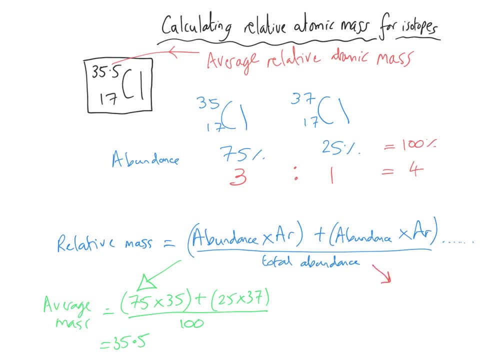 as it is in this instance, And so the sum that we'd do here would be the same principle. We'd do three multiplied by 35, and we'd add to that one times by 37, and instead of dividing by 100,. 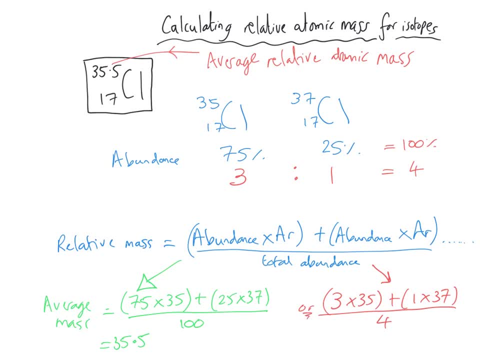 we'd divide by four and we'd get the same answer of 35.5.. And good to note, by the way, three significant figures, Or the number of significant figures that you've been given in the question. But if in doubt, 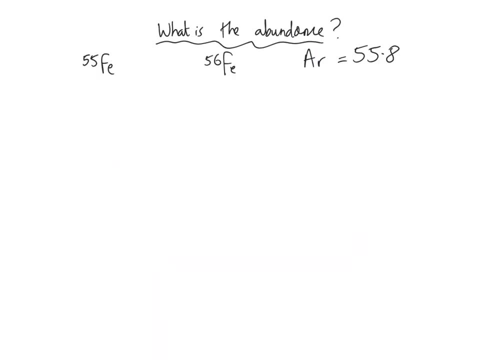 three significant figures is a good rule of thumb. And the last aspect of isotopes and their masses is: what about if they don't ask you what the average mass is? but what if they give you the average mass? And so you can see here: 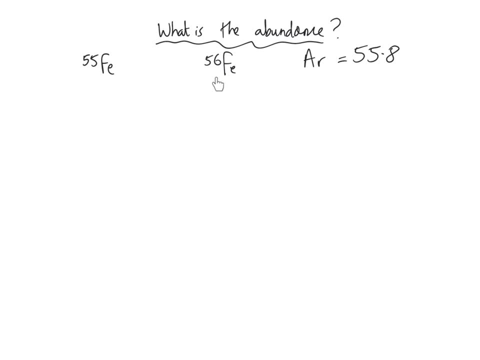 that we've got. the mass of iron is 55, but there's another isotope that's got a mass of 56, and the relative atomic mass is 55.8.. So that is the average on here. Now there's two different ways to do this. 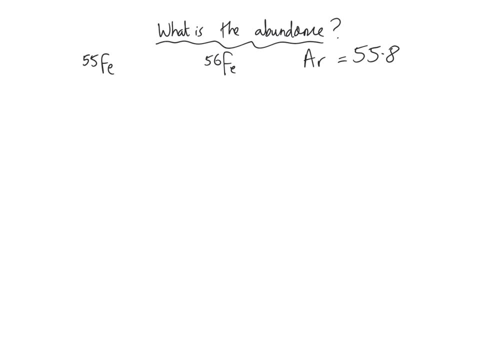 I'm going to show you the one that I think is the easier way first, and I think it's faster as well, And that seems a bit weird, but I'm going to make a number line and I'm going to put 55 at one end. 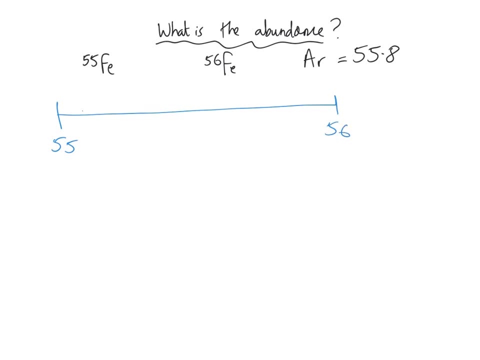 and I'm going to put 56 at the other end And I'm going to divide the rest into one, two, three, four, five, six, seven, eight, nine chunks, and I'll split it into 10 by dividing it nine times. 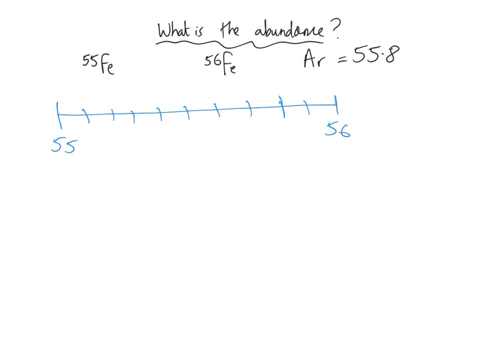 And so what we're going to do is we need to mark on 56,, 55.9,, 55.8 on there, And then how we use this number line is we take steps from one end towards where the average is. So this is the average on here. 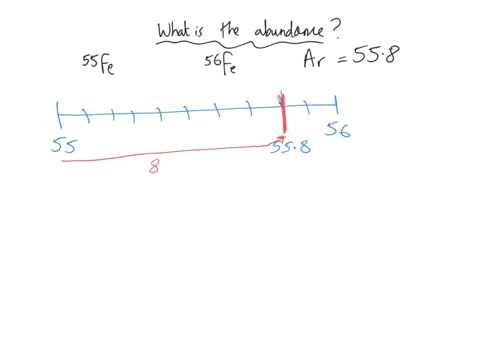 And we've split it into 10 chunks, and so we've moved eight out of 10 chunks, eight out of 10 steps towards 56. And what that means is eight out of 10 atoms of iron are 56. So this is 80% Fe- 56.. 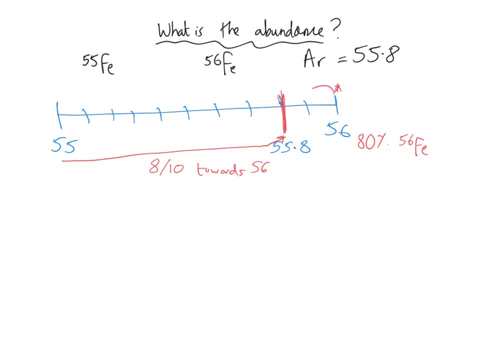 And if we start at the other end, if we start here and we go one, two, we take two of the 10 steps towards 55, and that tells us that it's 20% iron 55. Alternatively, if we had a look, 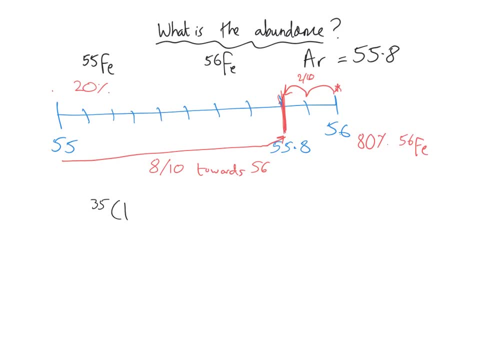 at the chlorine example from before. we've got chlorine 35, and we've got chlorine 37, and we don't know what the abundance is, but we know that the average is 35.5.. We could split it this time. 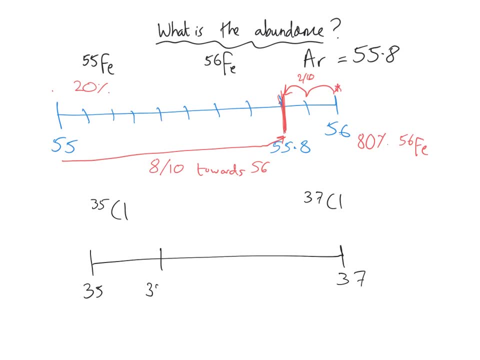 We don't always have to split it into 0.1. We split it into whatever makes sense, And so that's 35,, then 35.5,, that's 36, and that's 36.5.. So I've split this into four chunks this time. 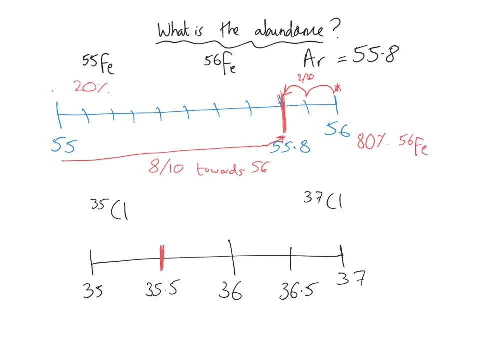 and the average is here 35.5.. So we've got quarters. We move one quarter of the way towards chlorine 37. And that tells us that one quarter of all of the chlorine is chlorine 37. If we started at the other end, 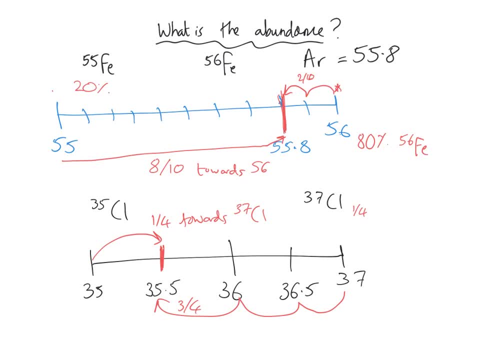 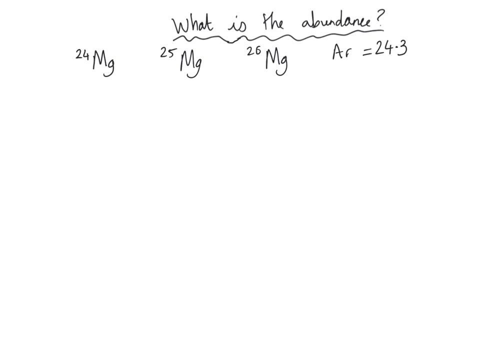 we move one, two, three quarters of the way towards chlorine 35. And that means it is three quarters chlorine 35.. Last of all, this question. you could solve this using a number line, but I think it's probably a bit easier not to. 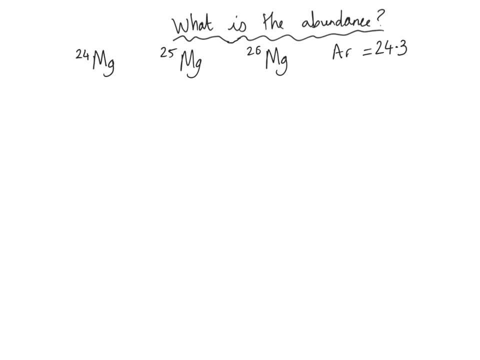 on this occasion, And so this question would say: magnesium exists as three isotopes: magnesium 24,, 25, and 26.. The average relative atomic mass is 24.3, as shown there, And they'd give you one fact. 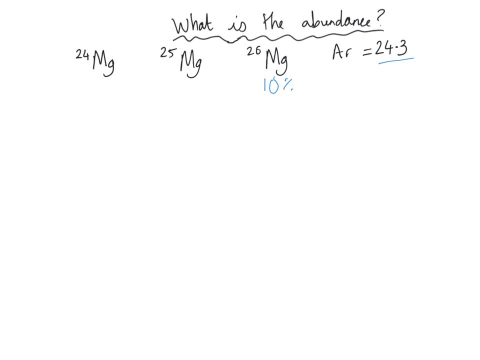 They'd say right, magnesium 26 is 10%. What is the abundance of the other two? Now to solve that, it's very easy to go down the wrong path in terms of maths and start trying to do a quadratic equation, And I really, really wouldn't do that. 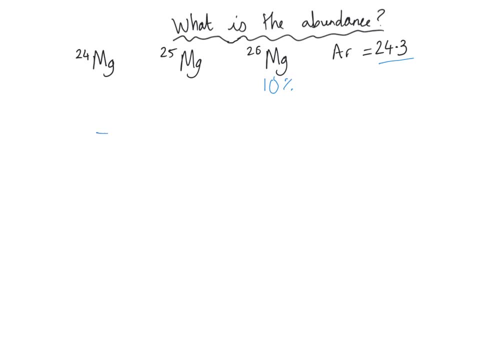 What I would do is I would set out the equation as you would expect to set it out. So we've got the abundance of magnesium 24, which we don't know what it is, So we're going to call it x And we're going to multiply that by its mass. 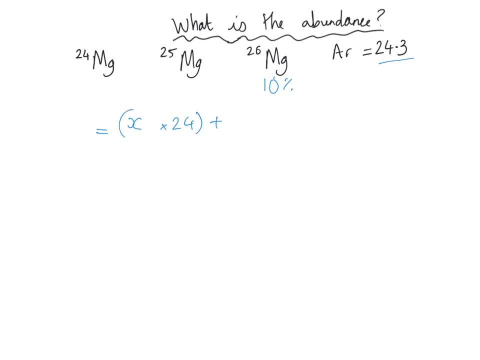 which is 24.. And we're going to add that to the magnesium 25.. Now this is where you could go down the quadratic pathway by putting a y in there and multiplying y by 25 and then adding to that 10 times by 26.. 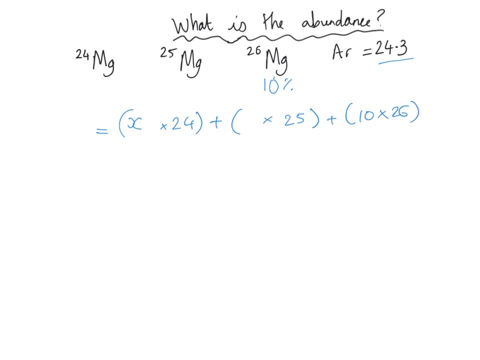 That's on the top axis, But what you have to remember is, of course, that percentages add up to 100.. And so if we've got 10% of magnesium 26 and we've got x% of magnesium 24,, well, the total is 100. 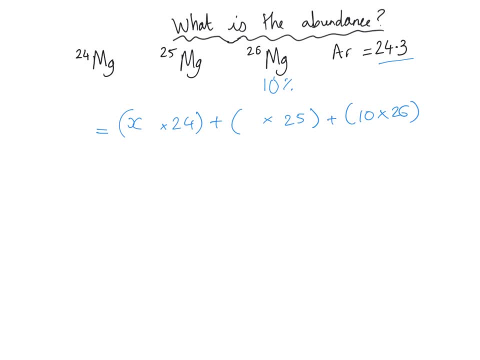 And so this is going to be, and we've used 10, and so this is going to be 90. take away x. We still don't know what x is, but we know that it is going to be whatever is left from 90. 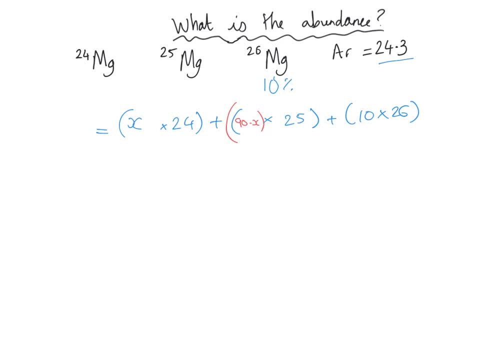 once you've taken x away is going to be our magnesium 25.. So let me just draw that in a quick pie chart so you can see what I mean. So we've got 26,, which is that section, And we've got the rest. 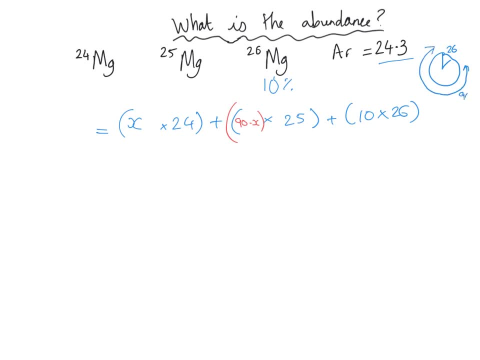 which we don't know what it is, but we know it is 90%. And so if we have got 25 and 24, that's going to be x and this is going to be 90. take away x On there And then we go back to what we know from before. 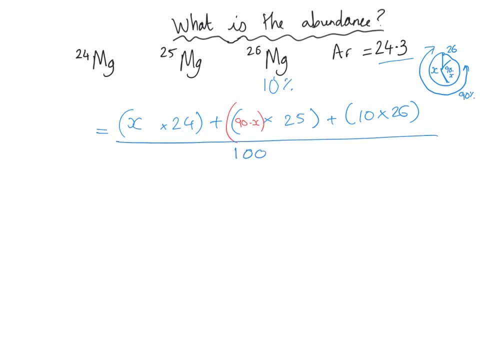 because we're working with percentages, so we need to divide all of this by 100.. What's different this time, of course, is we know what our answer is, so to speak. 24.3 is the average on here, And now we've set up this. 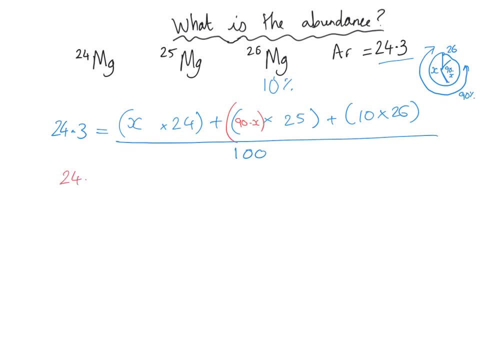 our final job is just to rearrange this, And so we've got: 24.3 multiplied by 100 is equal to 24x plus 2,250, which is 90 multiplied by 25, take away 25x plus 260 on there. 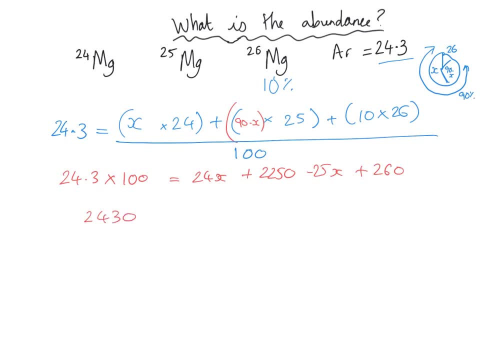 And then this, of course, gives us 2,430 on the left-hand side, And then this simplifies down to 2,510, take away x on there, And so if we move x over to this side, we've got x equals. 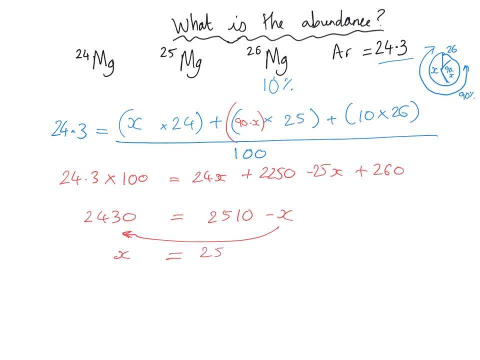 and then we take away the 2,430 from both sides, we get 2,510,. take away 2,430, which is 80%, which means the percentage of magnesium-24 is 80% up here. If the magnesium-26 is 10%. 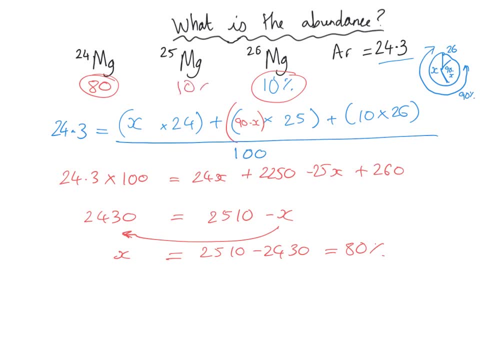 that gives us 90%, which means our magnesium-25 is 10% at the end. So we've worked out our two unknowns of 80% and 10% on there. Okay, that's everything. That's the whole of one topic.